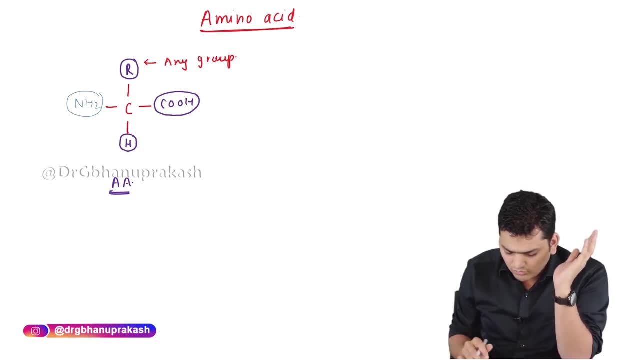 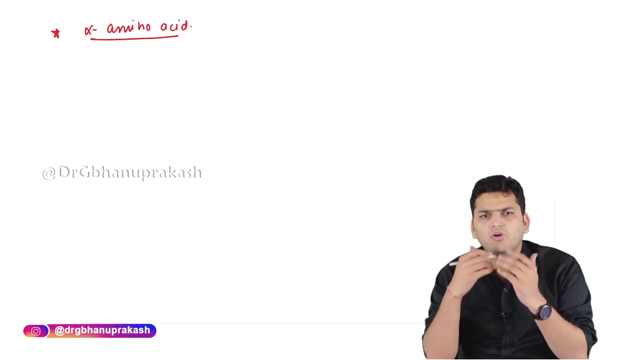 will make a base for this chapter of amino acid, right? So let's starting with. the first definition that we should know is alpha amino acid, Alpha amino acid. So to understand this alpha amino acid, we need to understand that. what is the meaning of alpha right? 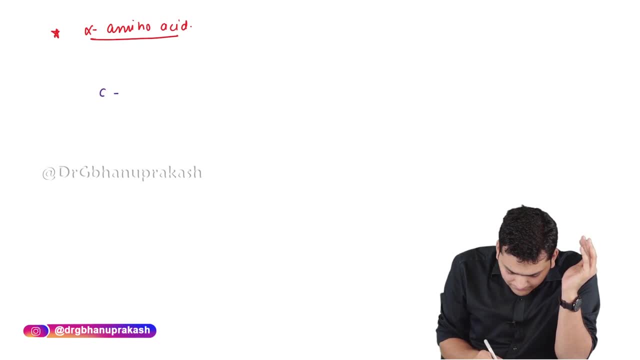 So to make you understand that I am taking a just simple example, Let's say this is a carbon chain and having the carboxylic acid as a functional group, right? So if I want to do the carbon numbering, we always start the carbon numbering from the functional group. So here is. 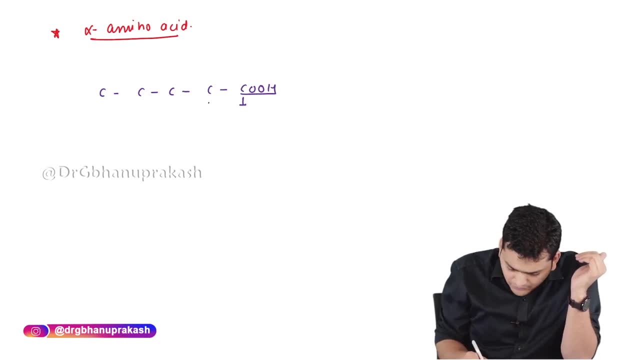 the functional group. So we will start with the carbon numbering from here. It's carbon number 1,, 2, 3, 4 and so on. right, This is one of the way of doing, carbon numbering The other way of doing. 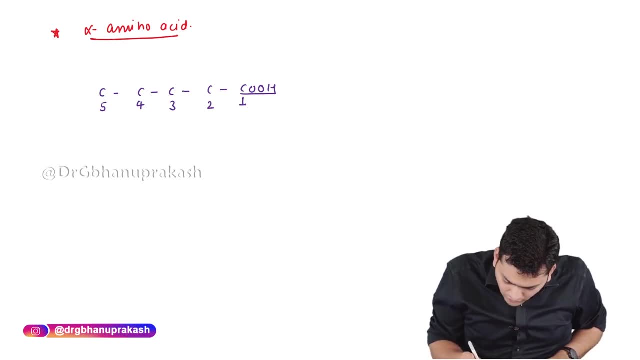 carbon numbering is that the carbon which is next to the functional group- Say, this is the functional group- is referred as the alpha carbon, Then the beta carbon, gamma delta, and so on. right, So what we have understood by this example is that what is alpha carbon is? 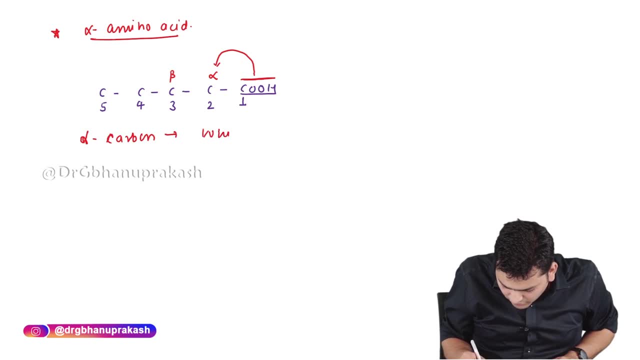 alpha carbon means the carbon which is next to the functional group, Carbon which is next to the functional group. The carbon which is next to the functional group is referred as alpha carbon If we apply the same concept of alpha carbon on the amino acid. 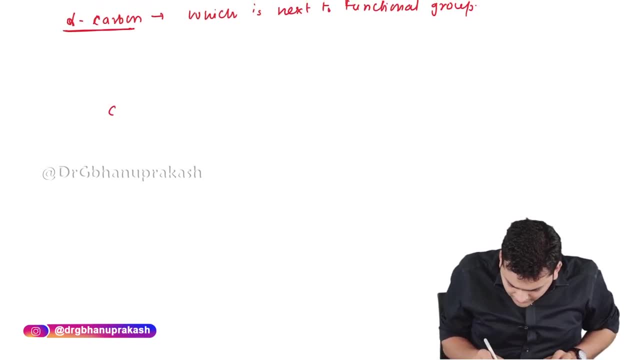 on the amino acid, then what we are going to appreciate is say this is the carbon having four valences. One valence is having amino group. Another valence is having acid group. The third valence is hydrogen. The fourth is can be anything from vitamin R. So this is a structure. 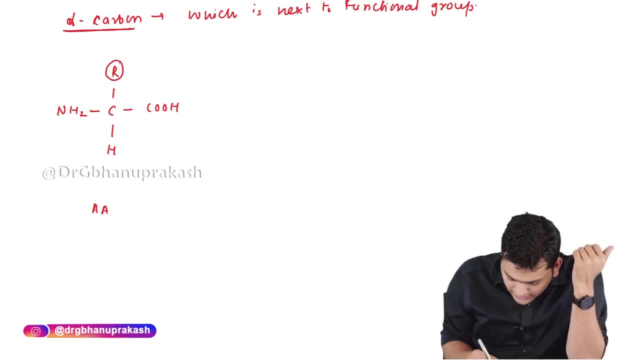 of amino acid. structure of amino acid. Because here is the main functional group, that is, the COH. Then the carbon next to the functional group, the carbon which is next to the functional group, is going to be the alpha carbon, is going to be the alpha carbon In this alpha. 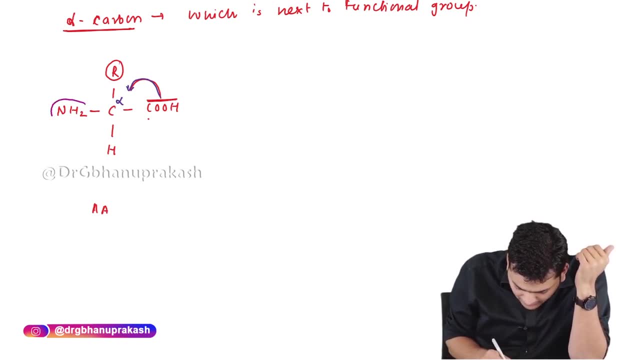 carbon. you can easily appreciate that this amino group is right now attached, right now attached to the alpha carbon. In this amino acid, the amino group is right now attached to the alpha carbon. So this is referred as alpha amino acid. This is referred as: so this is referred as the alpha. 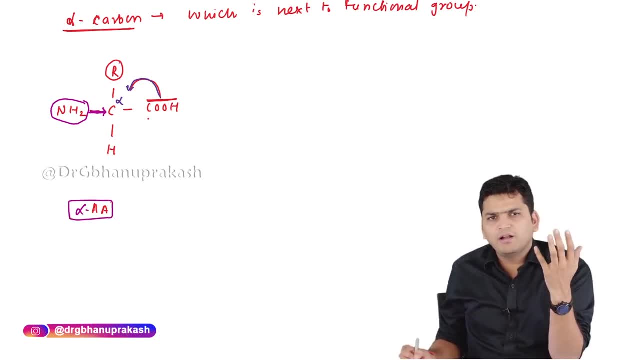 amino acid referred as alpha amino acid. So what is alpha amino acid? is that the amino group is attached to the alpha carbon. So let's write down the definition of alpha amino acid: that the amino group, amino group, is attached to alpha carbon. If the amino group is attached to the 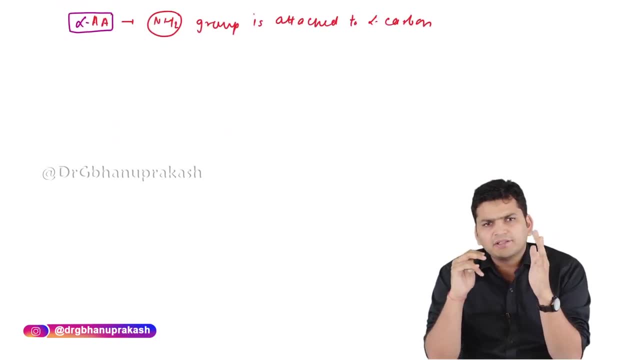 alpha carbon, that is referred as the. what happens in our body is that the most of the amino acid are found in alpha form. Most of the amino acid are found in alpha form. There are amino acid which is not found in the alpha form, and this is what we need to know. So the exceptions to the alpha amino acid means the amino acid which is not found in the alpha form. Exceptions to the alpha amino acid say they are beta alanine, beta alanine, beta alanine. the name itself is very clear that the amino group is attached to the beta carbon, that is, beta. 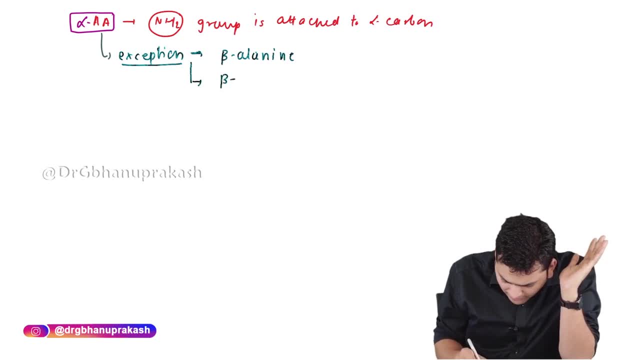 alanine. One more exception that we can add is beta amino isobutyrate, Beta amino isobutyrate, gamma amino isobutyrate. So the name itself is very clear that we have a prefix that beta alanine, beta amino isobutyrate, gamma amino isobutyrate, that the amino group is. 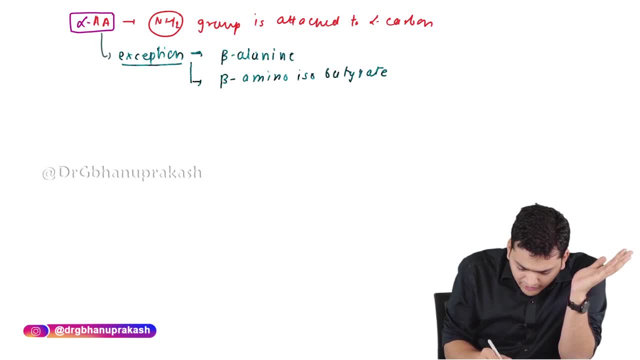 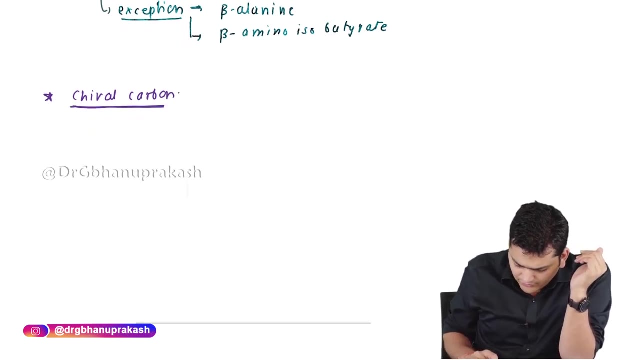 not attached to the alpha carbon. So this is the first definition that we need to remember in respect of the amino acid, that is, alpha amino acid. Let's understand the second definition, that is, with the name of chiral carbon: Chiral carbon. Now, what is the meaning of chiral carbon? 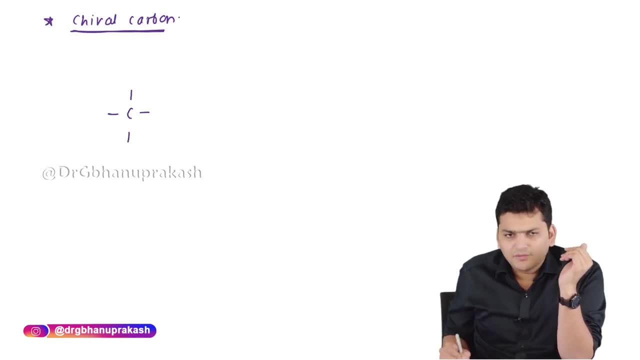 Is if we know that carbon have four valencies. carbon have four valencies. if all the four valencies are having different functional group- For example, here it is X, Y, Z, A- What you can appreciate is all the four valencies are different. If all the four valencies are different, then such: 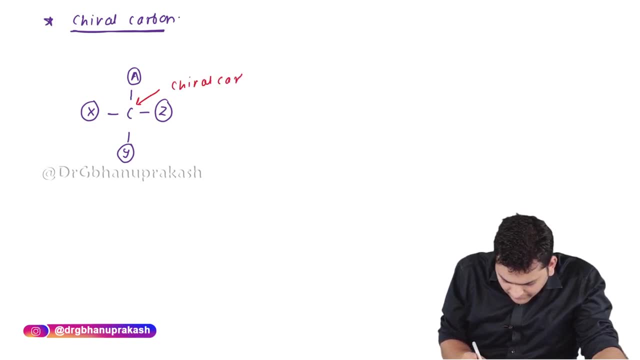 carbon is referred as chiral carbon. This is referred as chiral carbon. So what is chiral carbon? Definition is all the four valencies, All the four valencies having different functional group or different atoms. That is referred as chiral carbon. Now why this chiral carbon is important. See, you may have heard that something. 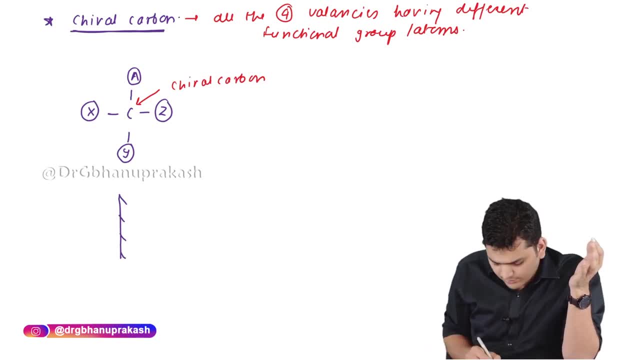 called, as there is something called as mirror image, There is something called as mirror image or the optic isomers. Mirror image or the optic isomers: If you want to make a mirror image of any molecule, the mirror image or the optical activity depends whether the molecule contains a chiral carbon. 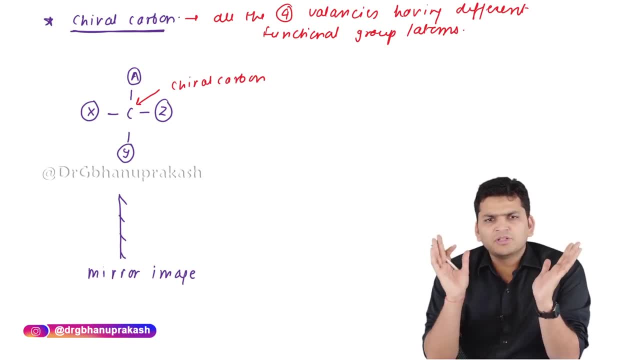 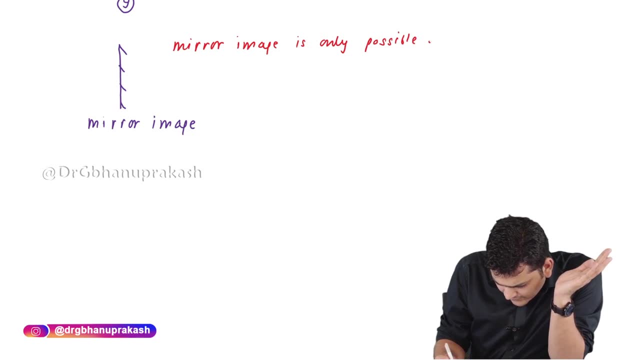 or not. If the molecule does not contain a chiral carbon, then the mirror image is not possible. So it is only possible if the molecule contains chiral carbon. If the molecule does not contain chiral carbon, then the mirror image is not possible. 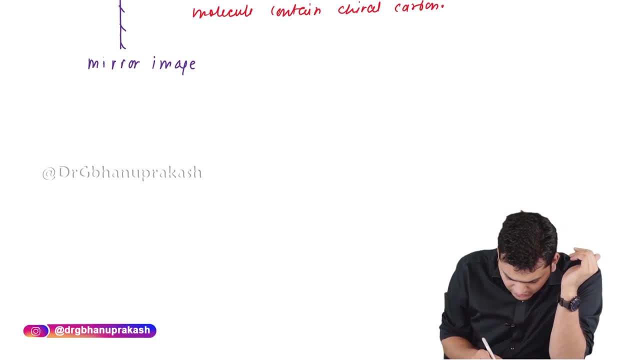 So, using this information, if I apply this concept here, on this structure of amino acids, here is the amino group and the acidic group. So this is going to be Amino acid and third valency is Hydrogen. Let us see the 4th valency is also Hydrogen. So what you can appreciate. 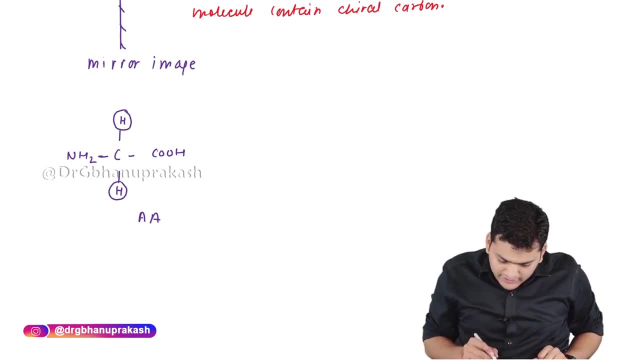 is third and fourth valency are same because two valencies are the same. So I can say it is not a chiral carbon. It is not a chiral carbon. Now let us consider this as a cuD63.. What is the value of the 4th valency of hydrogen? This is Malnutrile 3 and 4.. So the information. 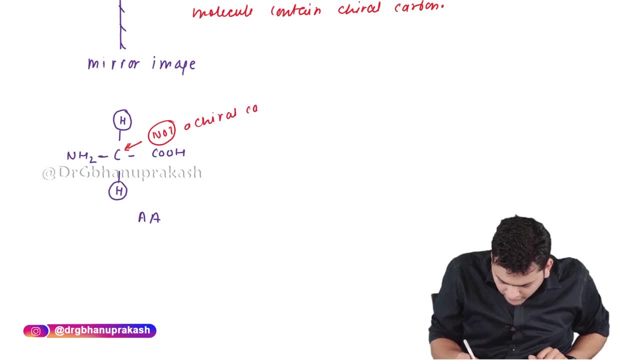 which we are gonna show what is thevoyance of amine acids is going to be. we have 2 values which accesses each valency and we put its is not a chiral carbon. now, once it is not a chiral carbon, once it is not a chiral carbon. 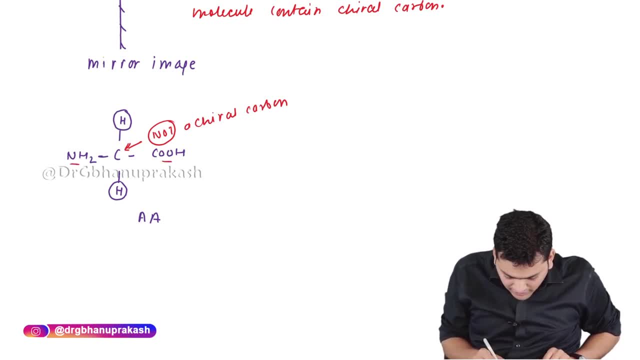 but at the same time it is having the amino group- acidic group- so it is amino acid. the name of this amino acid is glycine. so what they ask is which amino acid does not contain chiral carbon? that is a straightforward question. the answer is going to be glycine or in other way they can ask this. 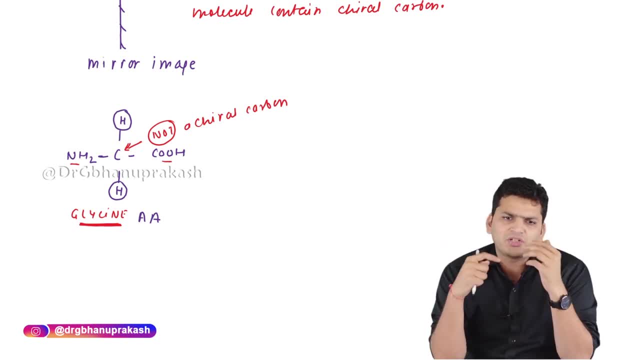 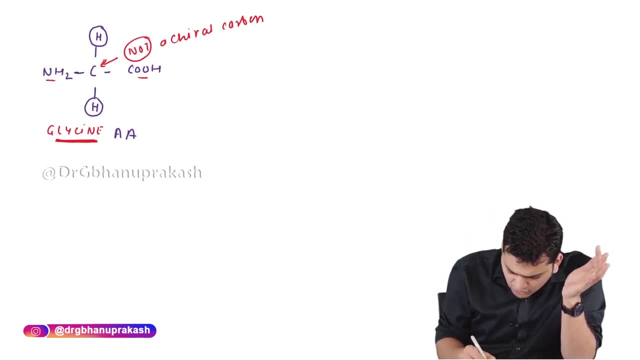 that which amino acid is optically inactive means which cannot make the mirror image. the answer is going to be glycine, because it does not contain the chiral carbon. so let's write down this point: that glycine does not contain chiral carbon, hence it is optically inactive glycine. 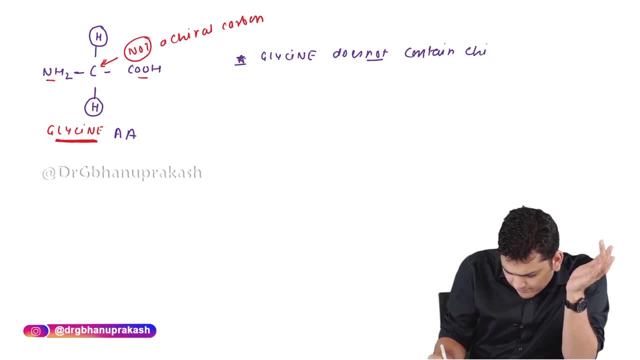 does not contain chiral carbon, hence it is optically inactive. does not contain kill carbon, so it is optically inactive. this is the second definition. the third: the third definition that we should know is: the third definition that we should know is amino acid. so we have discussed about alpha amino acid, then the kyl carbon. the third: 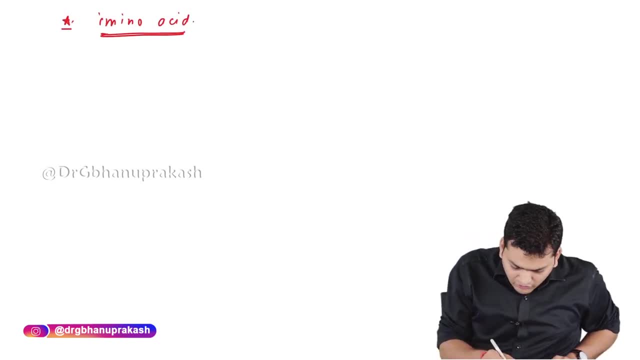 that we are discussing is amino acid. if i make the structure of amino acid, carbon, having four valencies on one of the valency we are having, the amino group, the acidic group, the hydrogen, and the fourth valency can be anything. so identity r now here. what you can appreciate is that the amino group is free, in a sense that it can make bond. 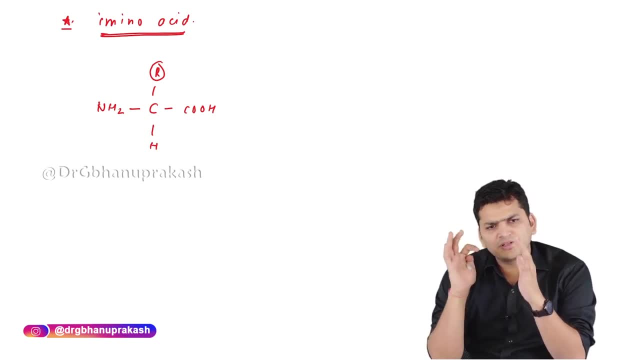 with the nearby amino acid. it can make peptide bond with the nearby amino acid. it is currently free. this amino group is free, but what i do is, if i alter the structure of the amino group means right now this amino group is free, but now what i do is i bound this amino group in a ring. 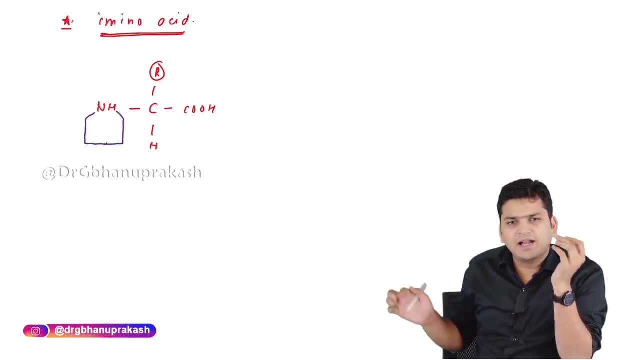 structure like this. now you can see that i have made a ring around the amino group, right? this amino group is not free. if the amino group is not free, then this molecule is referred as amino acid, referred as amino acid. so what is amino acid? that the amino group is not free? 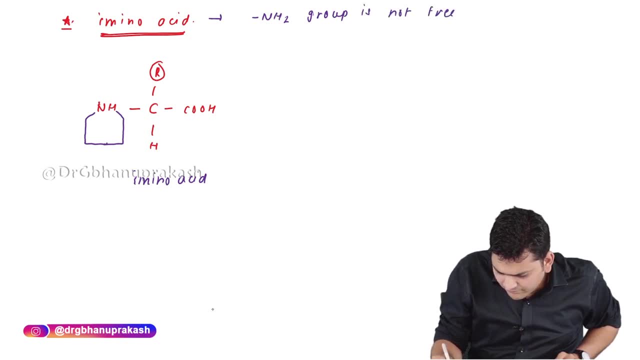 is not free. instead, it is bound in a ring structure. in bound in a ring structure. if the amino group is not free bound in the ring structure is referred as amino acid. what is very important is that. what is the example of amino acid? the example of amino acid is proline. 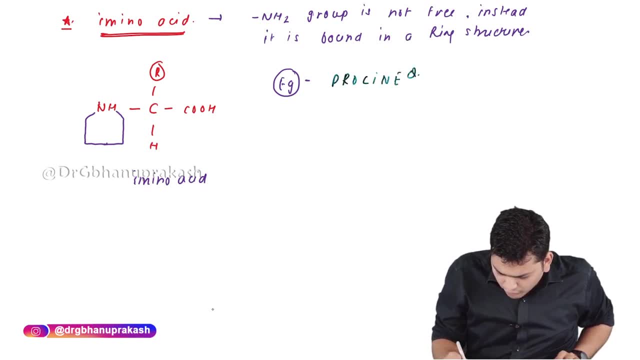 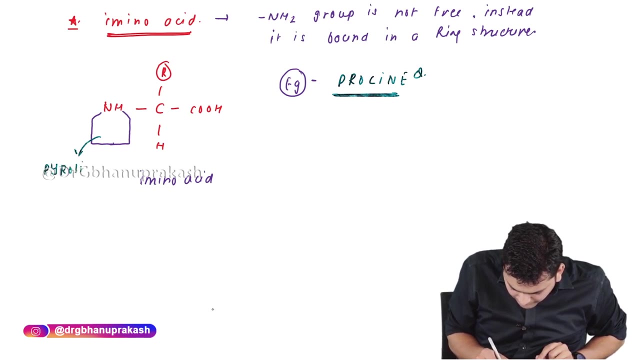 proline is the example of amino acid. it does not have the free amino group. sometimes they might ask that what is the name of this ring? what is the name of this ring? the name of this ring is this is referred as pyrrole, so pyrrole leading ring is found in which amino acids found in proline, which is an example of. 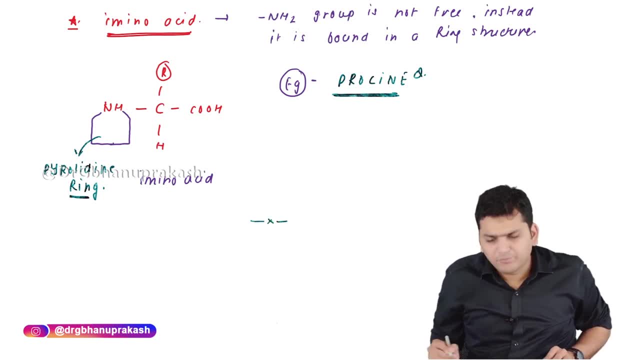 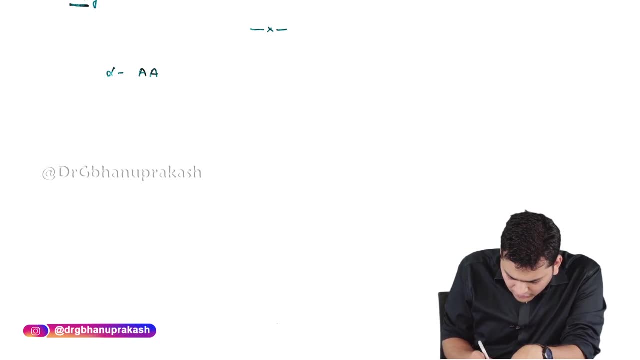 amino acid. so these are the three definition to be remembered, right? so to summarize what we have discussed, that the first thing that we need to know is the alpha amino acid. in humans, most of the amino acid are found in alpha. there are few exceptions, and the most important exception that 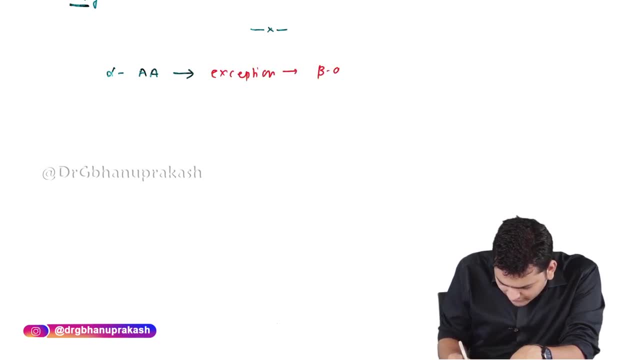 you should know, is beta alanine. now, when they will ask this question, they will not write this beta word in the options. the reason is, if they write beta, then it is going to be very obvious, right, so the beta, what they will remove, they will just write alanine. alanine is the example of beta amino acid, the, the second thing that we have. 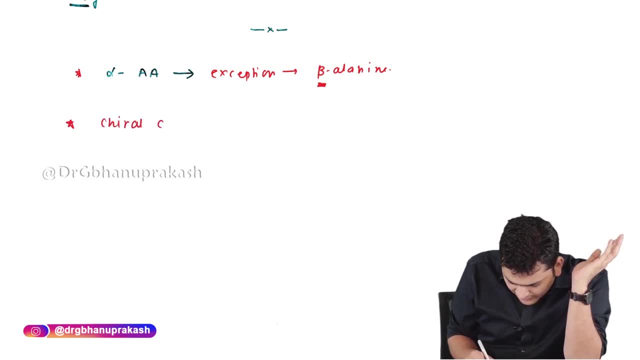 discussed was the chiral carbon, chiral carbon or the optical activity. so the point to be remembered is chiral carbon not found in which amino acid. the only amino acid is glycine, which does not have the chiral carbon. it is optically inactive. the third thing that we have discussed was amino acid. 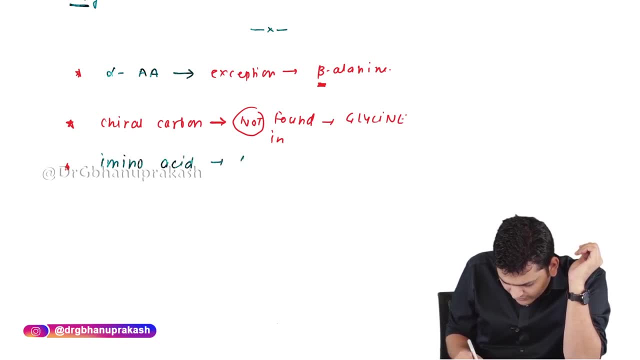 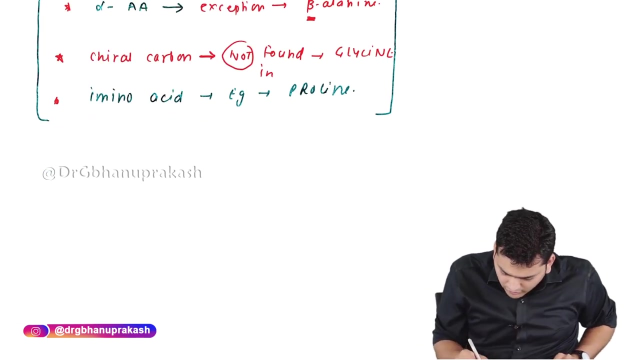 the example of amino acid is very important is proline. the amino group is not free, is bound in a ring structure. so these are the three points to be remembered from this definition part. now coming to the very important part of the chapter amino acid, and that is in respect of 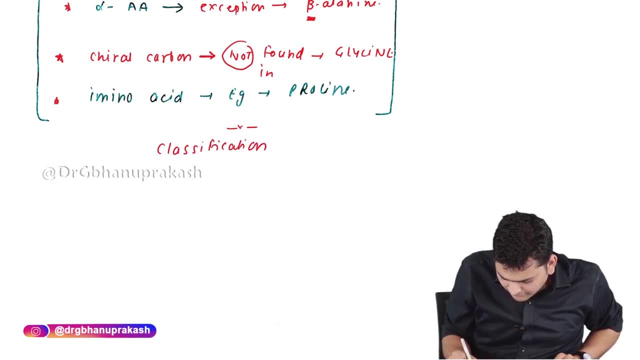 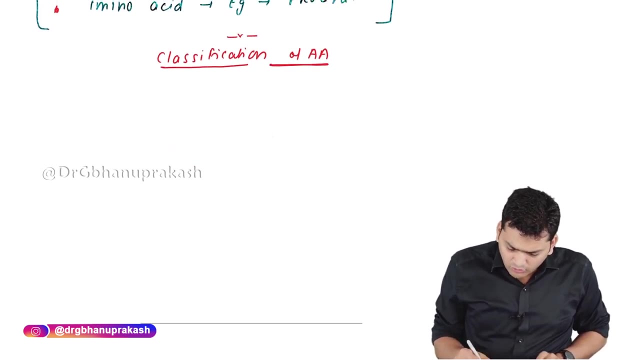 the classification of amino acid. classification of amino acid. so to do the classification of any group first, we need to understand that how many amino acids we have. earlier we have 20 types of amino acids. now, recently two more amino acids are added and now we have total 22 types of amino acids. 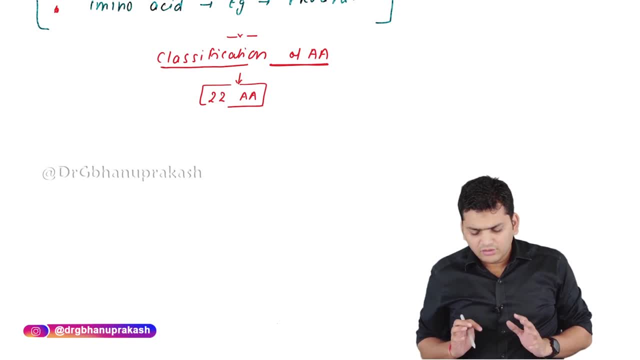 we have 22 types of amino acids and we need to classify these 22 group- uh, 22 amino acid. so to classify any group, any group, say, for example, if we are having right now 22 tiếng student in the classroom and i want to classify these 22 students. so what i can do is i need to. 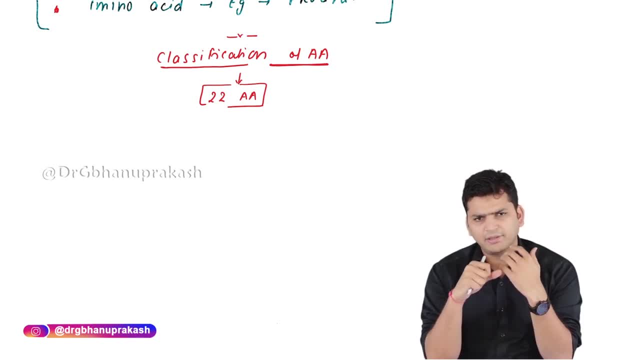 have a basis, on what ground i am going to do the classification. say, for example, i can do the classification on the basis of your age: 21, 22 year, 23 year, 24 year and so on. i can classify on the basis of your, let's say, the native state: rajasthan, gujarat, maharashtra, telangana, kerala, and so on. 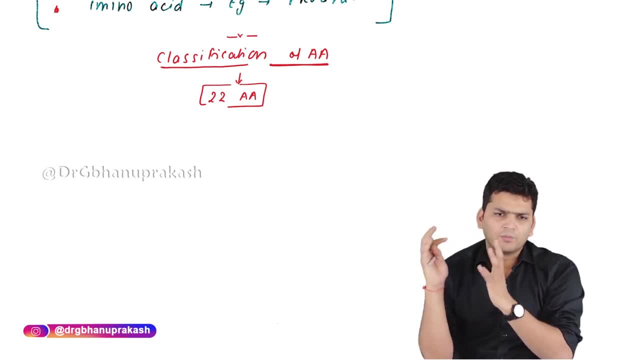 right. so on the basis of various thing we can classify the groups. so the here also we want to classify the amino acids. so first we need to understand that on what ground we are going to do the classification right. so the first classification that we are going to discuss. 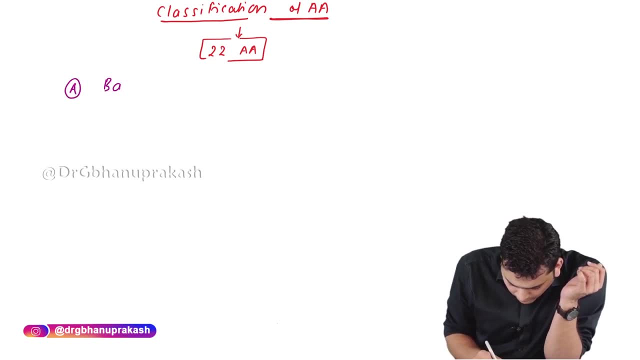 is based on the r group. based on r group. what is r group? r group is basically the side chain. if i make the structure of amino acid that we have made earlier, is the amino group acidic group hydrogen. the fourth was r. the fourth valency was r, as i told you. 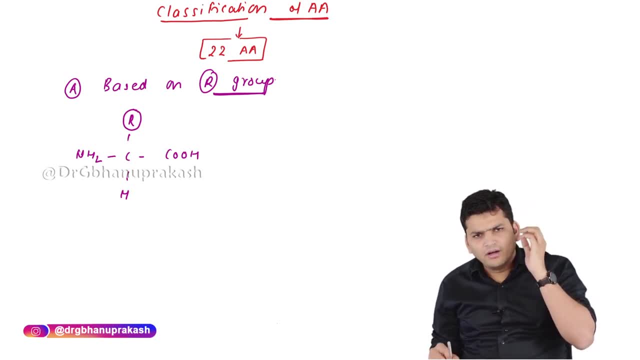 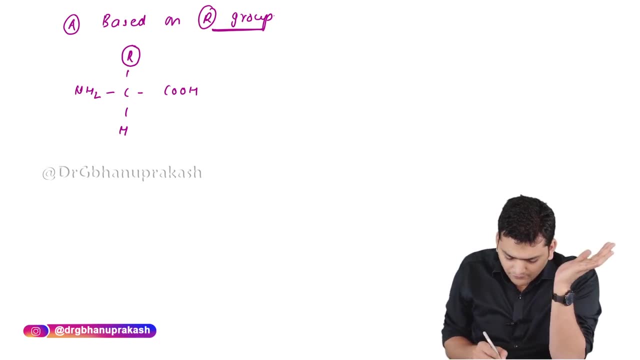 earlier that r can be anything. it can be hydrogen, it can be carbon, it can be sulfur alcohol, it can be anything. so based on that we are going to do the classification. so the first subcategory, the first subcategory, if we do the classification, that is based on the r group, the first subcategory. comes out to be simple amino acid. simple amino acid means that the r group is replaced by either a simple hydrogen or by a simple carbon. if you replace the r group with simple hydrogen or carbon, that is called a simple amino acid. the example of simple amino acid are glycine and alanine. glycine and alanine are the example of simple amino. acid. glycine is being the simplest amino acid among all the 22. the simplest amino acid is glycine. When it comes to alanine, alanine is the most abundant amino acid that is found in the body. Most abundant amino acid that is found in the body is alanine, right? So these are the two. 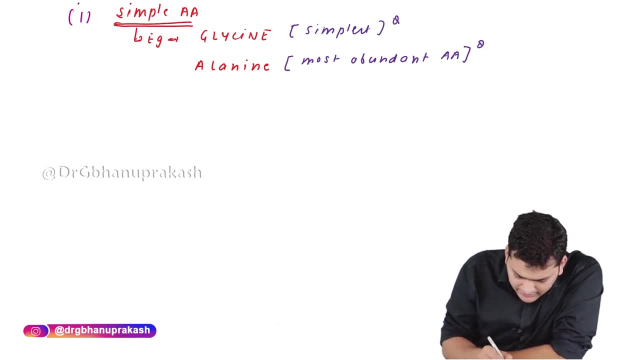 simple amino acid. that we have Coming to the second subcategory. the second subcategory is the branch chain amino acid. Branch chain amino acid means that the R group is replaced by a branch carbon chain. R group is replaced by a branch carbon chain that is called as branch. 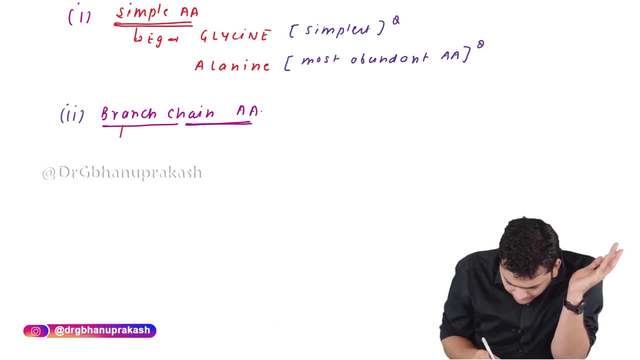 chain amino acid. The examples are leucine, isoleucine and valine. Leucine, isoleucine and valine- they are the branch chain amino acid. How we can remember? We can remember via mnemonic. that is, if you want to have a branch relationship, if someone wants to have a branch. 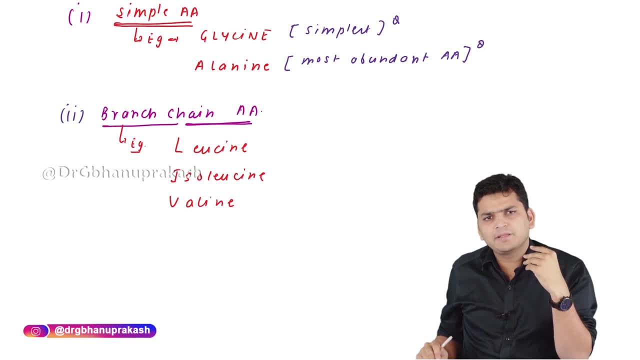 huge branch relationship. the person has to have a specific characteristic: that the person has to be live hearted. The person has to be live hearted. So what I can say is to have the branch relationship, to have the branch relationship, the person has to be live hearted. The person has to 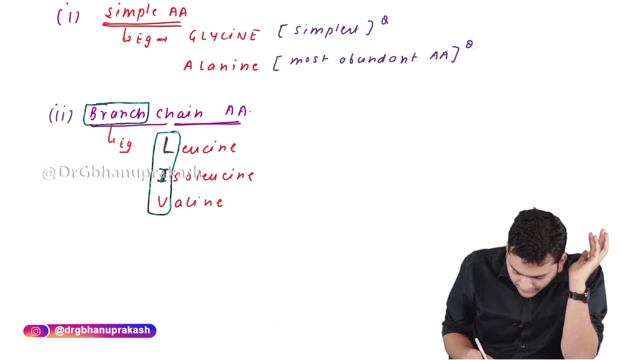 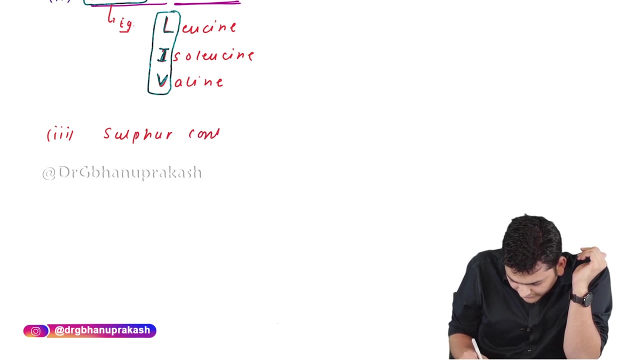 be live hearted: Leucine, isoleucine and valine L-I-V. To have branch relationship, the person has to live hearted. So what do you think about branches, chain amino acid, branch chain amino acid- Do they exist? According to meille divine sources, the key is behind branches which. 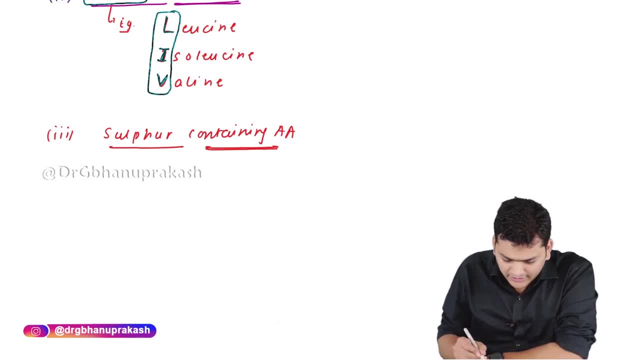 is the juniper on branches chain amino acid in the shape of a mnemonic means. they are the branches. This branch chain amino acid was like this: two branches, All branches are with l-I-V, This one, for example, with l-I-V, And here also branches are full of l-I-V. right. So here you can notice that he has two branches: One is Viral and the other available. There are three branches then. As I said, The first branch chain is complex and he is a branch working, But South American, This is a branch chain amino acid, Unlike mist, which does not connect with food. acid, so it will remember it. methionine and cysteine, we can remember like this, methi cyst- methi means sweet. what is there inside the methi cyst? it is the sulfur. what is there inside the methi cyst? it is sulfur. methi cyst, the fourth. 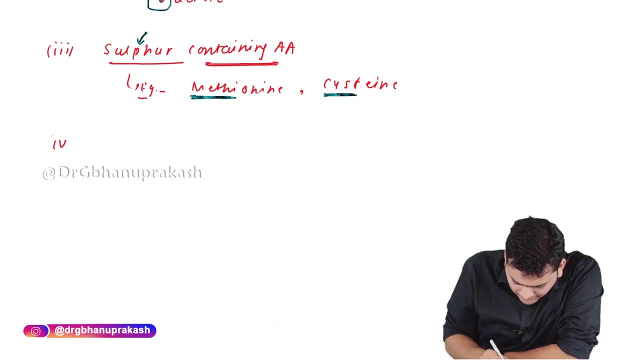 subcategory, the fourth subcategory. it is the hydroxyl group containing amino acid. hydroxyl means alcohol a OH. OH means the hydroxyl hydroxyl group or the alcohol group containing amino acid. alcohol group containing amino acid. hydroxyl group containing amino acid. the examples are: the examples are serine: 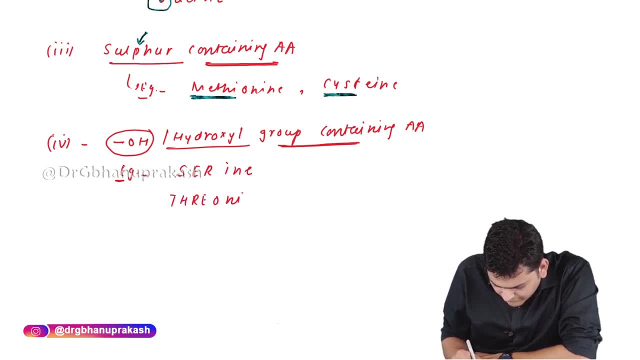 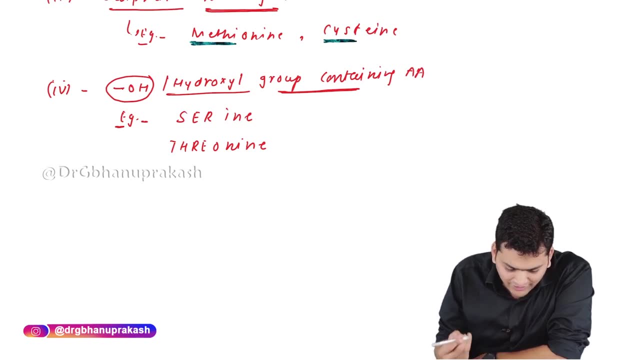 threonine, serine and threonine. these are the examples, how we can remember it. how we can remember it, the example we can remember it is in Hindi. so if you know, we is very good, if not fine, you can remember it directly. seaweeds. 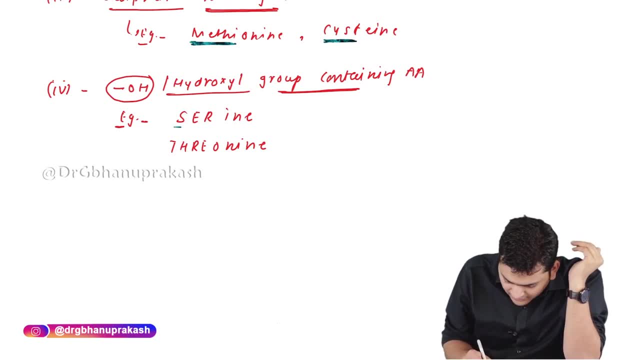 are serine and threonine. the mnemonic is: certaro, this is alcohol. certaro, this is alcohol. certaro, certaro means stop, certaro D is alcohol. that is serine and threonine. these are the two amino acid which contains the hydroxyl group. but then, the interesting thing, part of this, mencionned hydroxyl group. but there is another student of mine. he has LPT and he he has plasma. so he just one. Cuando esta haciendo una zona de Помp During the Donon, hoềте referr: "-лагa-nos en whisd medication. may you убий trafico". 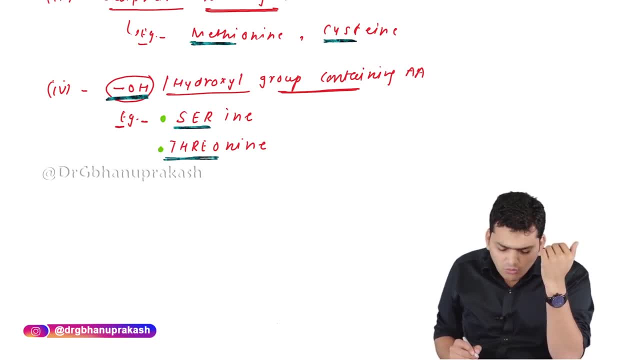 is one more amino acid apart from these two. there is one more amino acid which also contains the hydroxyl group, but there is certain characteristic difference between these two and the third one, right, so that is why i have not, uh, told that earlier. i told that hydroxyl group containing 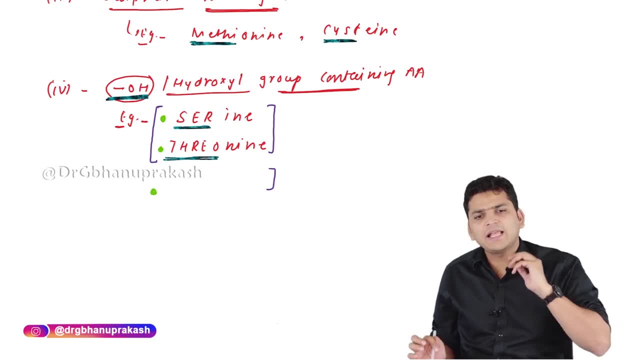 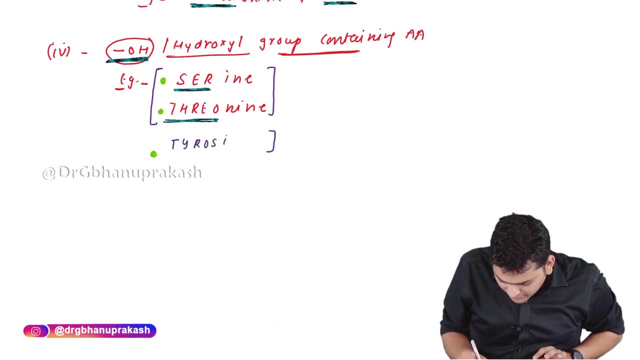 you need to remember, to serine and threonine there is one more and that is having some different characteristic. let's first write down the name of that amino acid. the name of that amino acid is tyrosine. tyrosine also contains the hydroxyl group. tyrosine also contains the hydroxyl group. 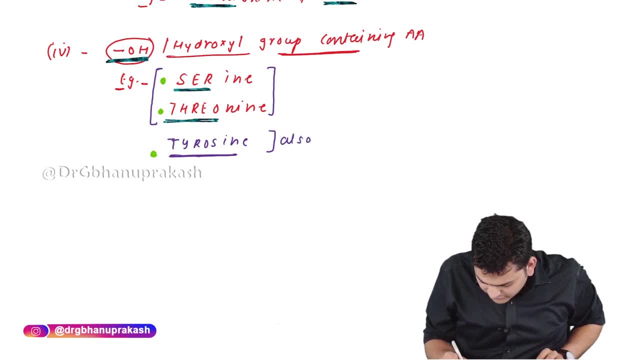 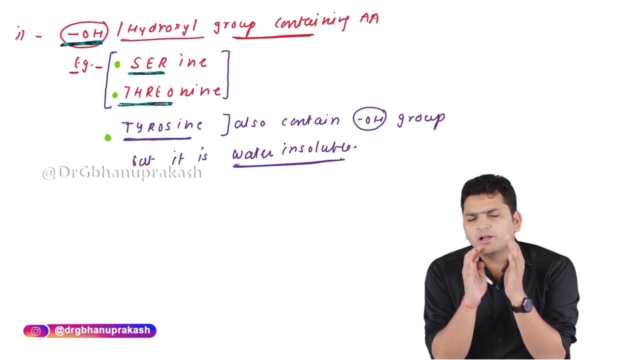 right, but let's write down this full statement: tyrosine also contains hydroxyl group, but it is water insoluble. but it is water insoluble. now, what is the meaning of that? see, usually what happens is that that that the alcohol containing amino acid are water soluble. We can easily understand that alcohol. 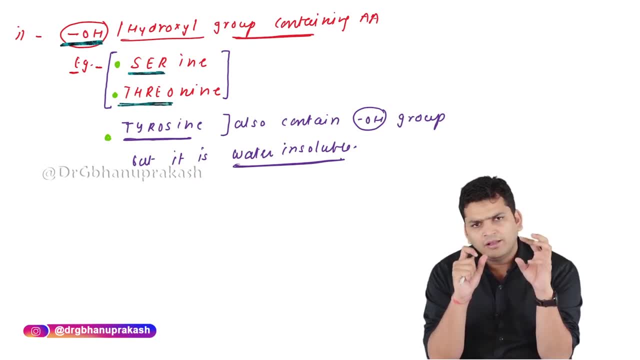 is water soluble. So wherever there is alcohol that is going to be water soluble. So the alcohol containing amino acid are water soluble usually, and that is serine and threonine. Tyrosine, despite it, contains hydroxyl group but it is not water soluble. That is why we are writing that in a 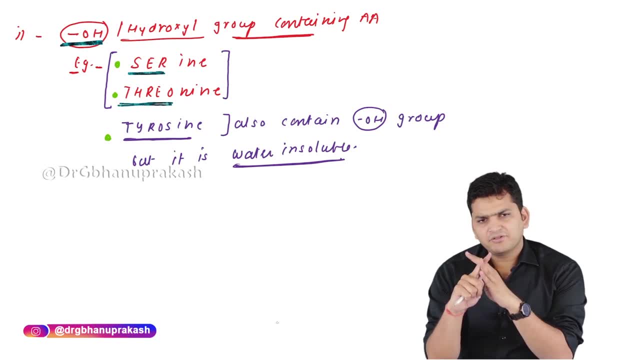 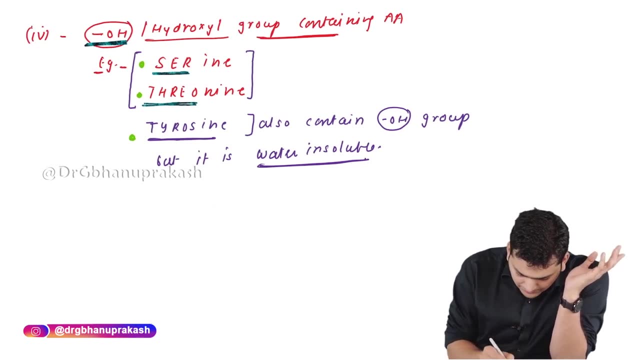 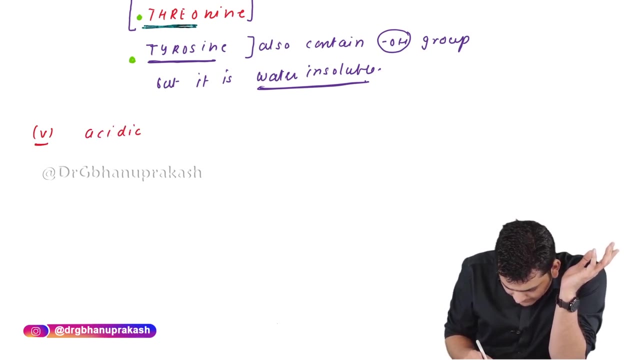 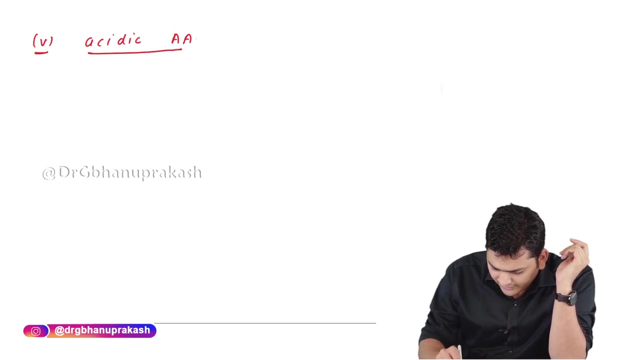 separate line. So the alcohol containing serine, threonine, tyrosine, Tyrosine, we are writing in a separate line because it is hydrophobic, It is not water soluble. Coming to the fifth sub-category, that is, the acidic amino acid. Acidic amino acid: We can write acid, like COOH, We can write acid. 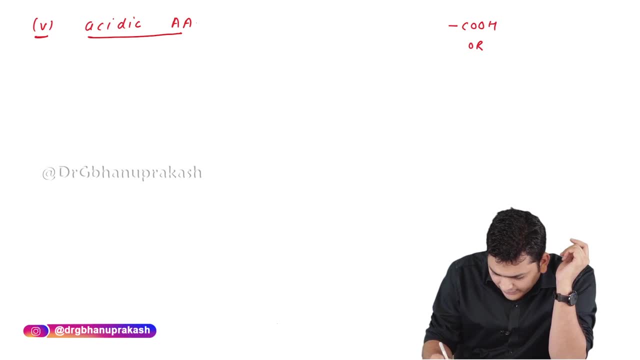 like COOH or we can write like COO negative. The point I want to convey to you is that wherever there is acid, there is acid. So we can write acid like COOH or we can write like COO negative. So wherever there is excess amount of acid, it may contain which charge It will contain which. 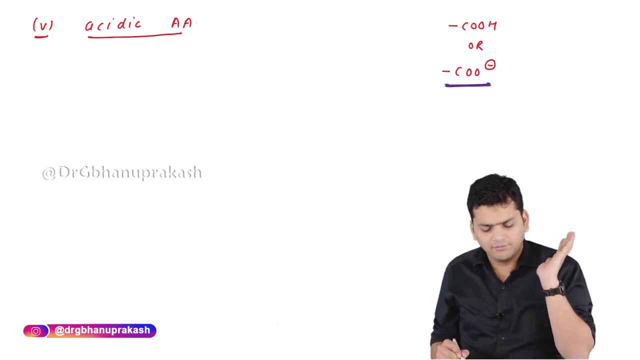 charge. Negative charge because you write COOH or COO, negative same. So wherever there is excess amount of acid, it is going to contain negative charge. So it is. these are the negatively charged amino acid. These are the negatively charged amino acid, The examples of the acidic. 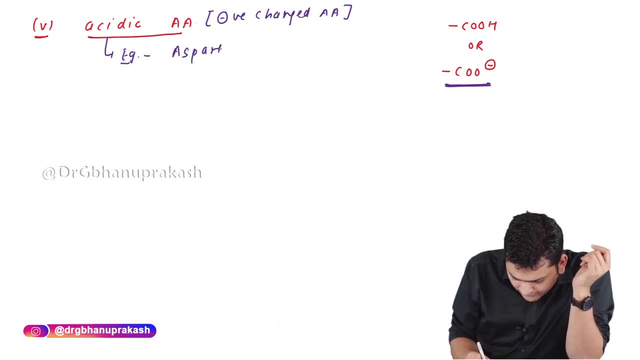 amino acid are aspartate and glutamate. Aspartate and glutamate. The other names of these aspartate and glutamate, is aspartic acid and glutamic acid, because when the examiner will try to ask you that which are which of the following is the acidic amino acid, they will 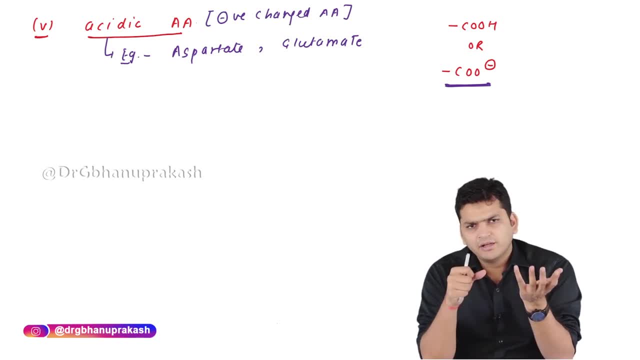 not give you the name aspartic acid or glutamic acid, because name itself is very clear, So they will use the alternate names: Aspartic acid, also called as aspartate, Glutamic acid, also called as glutamic. These are the acidic amino acid. The sixth sub-category is amide group. 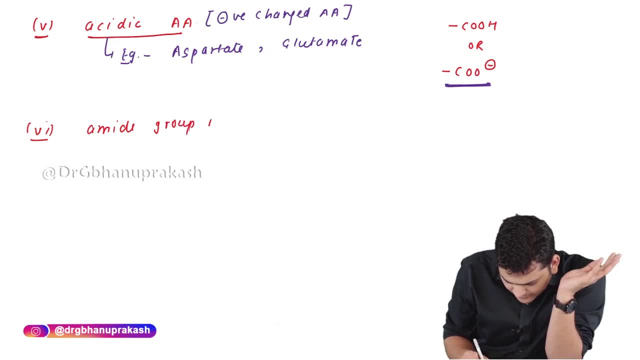 containing amino acid. Amide group containing amino acid. Amide group Containing amino acid. So to understand amide group containing amino acid, first we need to understand that what is the meaning of amide group is What is the meaning of. 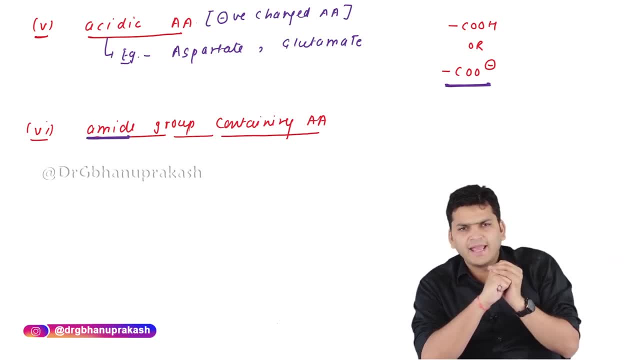 amide group. When I say it sulfur content, is very obvious that it is containing S. When I said hydroxyl group, we know it is OH. When I am saying that is amide group containing, first we need to see what is the amide group is See the amide group is CONH2.. 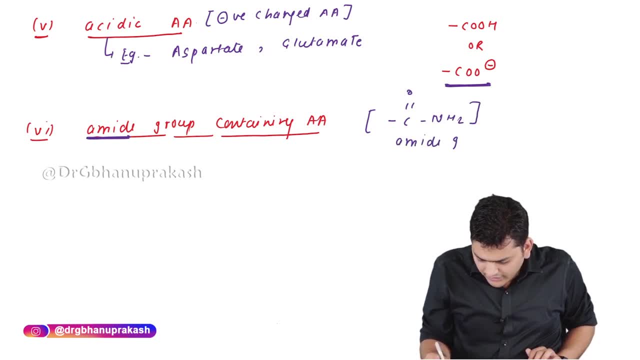 This is referred as the amide group. So we need to look for the amino acid which contains this amide group. This amide group has a tendency that it loves the acid. Let's understand it here. What I am saying is that the amide group has a tendency that it loves the acid Wherever. 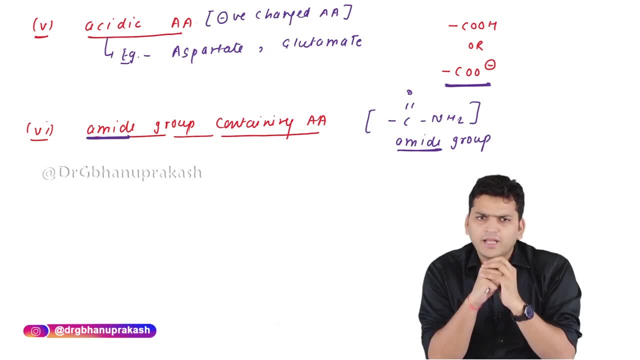 there is excess amount of acid, this amide will go and will attach on that. Just prior to this, we were discussing about the acidic amino acid. Acidic amino acid means that they have the excess amount of acid. So we have two amino acids which have excess amount of acid- aspartate and glutamate- And right. 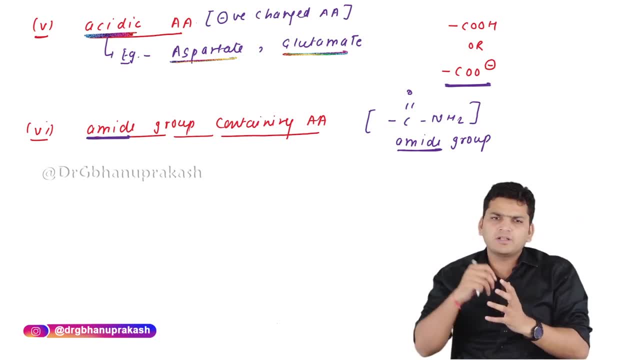 now I am saying that the amide has a tendency or affinity towards the acidic amino acid. So what is going to happen is that this amide is going to attach on the aspartate as well, as it will go and will attach on the glutamate. So the example, when it comes to the example, 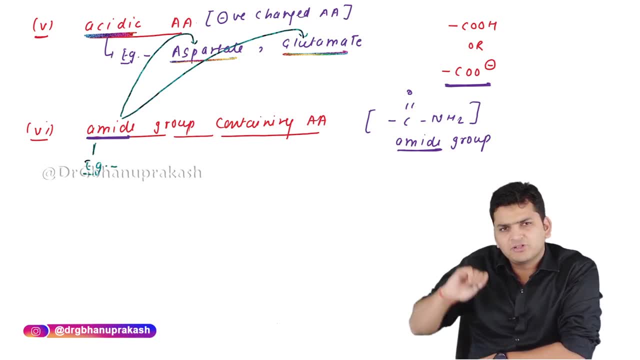 of amide group containing amino acid. I can see that amide will go and will attach on aspartate. It will make a molecule that is called as asparagine. If amide goes and goes and attaches on glutamate, it will make the molecule that is with the name of glutamine. 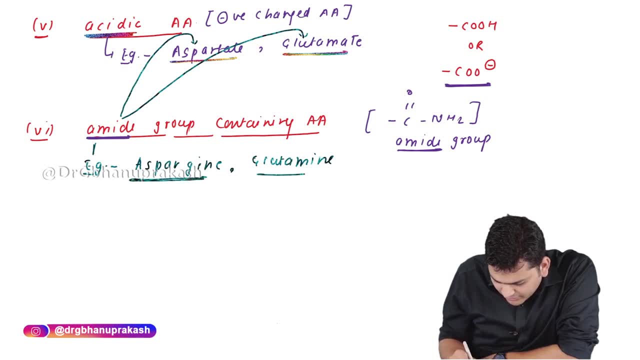 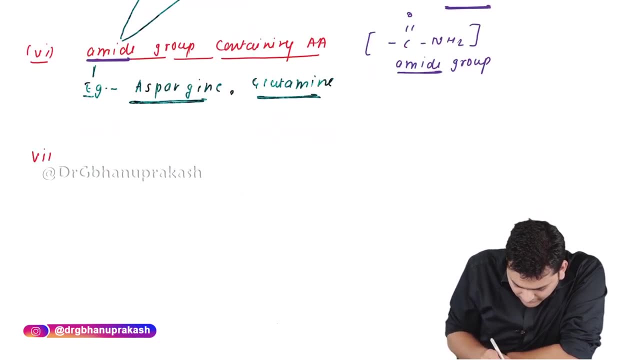 So we have understood that, the amide group containing amino acid. we have two: the asparagine and glutamine. Then the last subcategory I can see is the seventh one is the basic amino acid. Basic amino acid Basic means the I can see they have the excess amount of base. 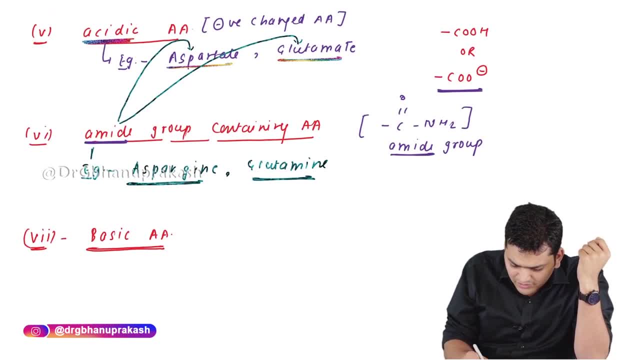 When I said the acidic acidic are heavy amino acids. So when I said the acidic acidic are having with charge, negative charge, If acid is negatively charged, the opposite base is going to have with charge, is going to be having the positively charged amino. 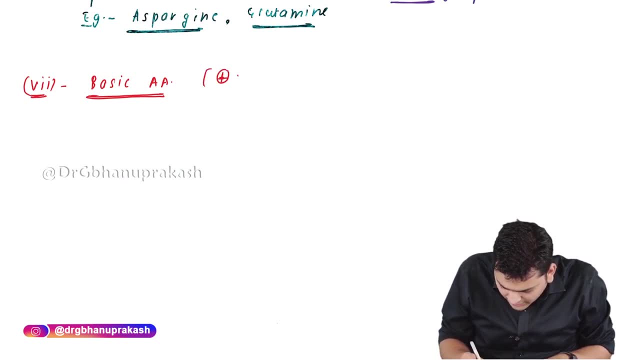 acid. So I can say basic amino acid or positively charged amino acid, positively charged amino acid. The examples are histidine, lysine and arginine. These are the basic amino acids: histidine, lysine, arginine. How we can remember is with the simple mnemonic: his last urge is very basic. His last urge. 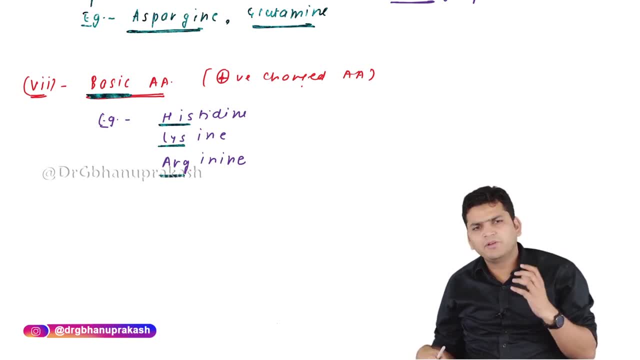 is very basic. Whenever it comes to last wish, it's going to be very basic. only His last urge is very basic. Among these three, if they ask that which is most basic, which is having the highest pH, the answer is going to be arginine. Arginine is having the highest. 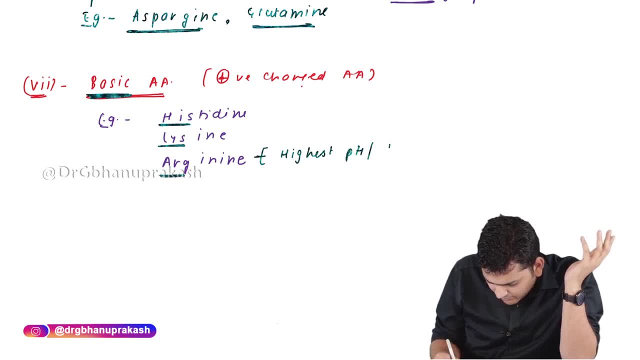 pH. Or in other words, I can say most basic. In other words, I can say most basic. So these are the seven sub categories of the amino acids based on their R group. Based on their R group: Simple bran chain, sulphur. 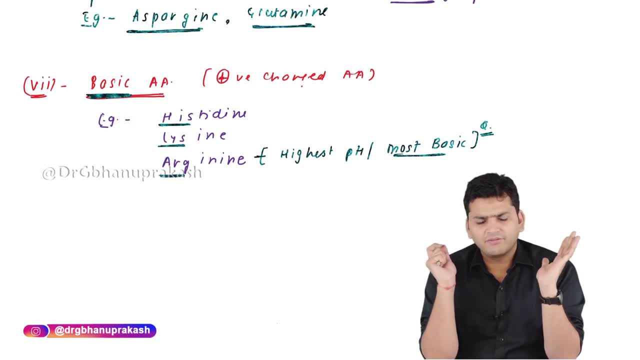 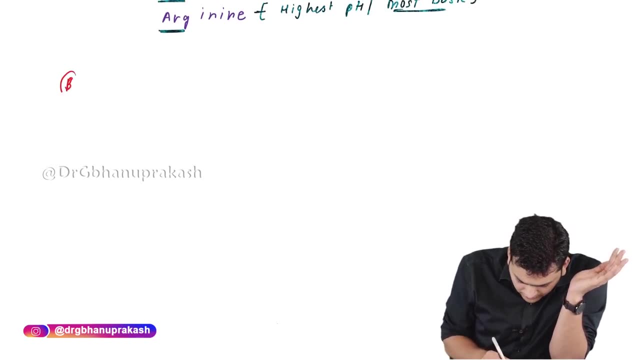 containing hydroxyl group. containing acid base and amide. These are the seven categories. The next classification that we are going to discuss is based on water solubility, Or I can say whether the amino acid is water soluble or not. right, so we are going to discuss the next. 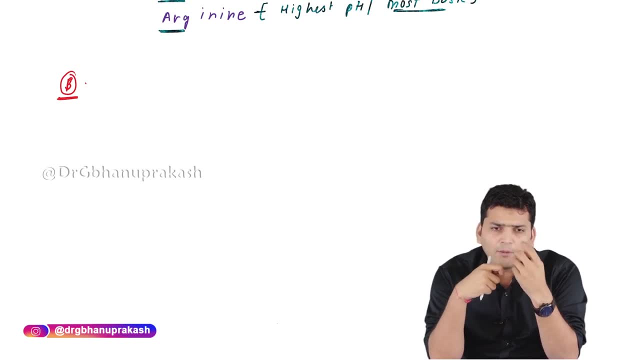 classification based on the the property of the amino acid, whether it is water soluble or not. right, so let's write down the second type of classification, that is based on water solubility. water solubility: based on that, we can divide the 22 amino acid into. 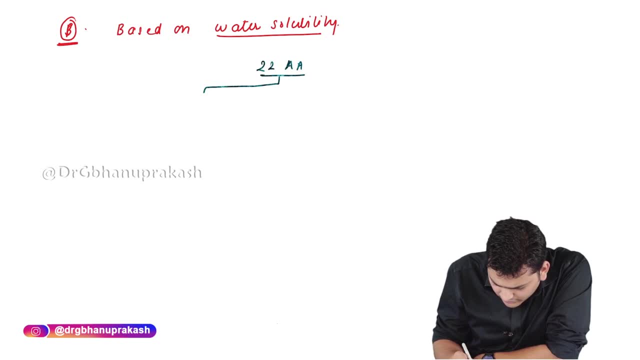 two categories. one is the water soluble, that is, the hydrophilic category and the hydrophobic category. hydrophilic and hydrophobic hydrophilic. they are also referred as polar amino acid. polar amino acid or hydrophilic is seen. polar or hydrophilic is seen when it. 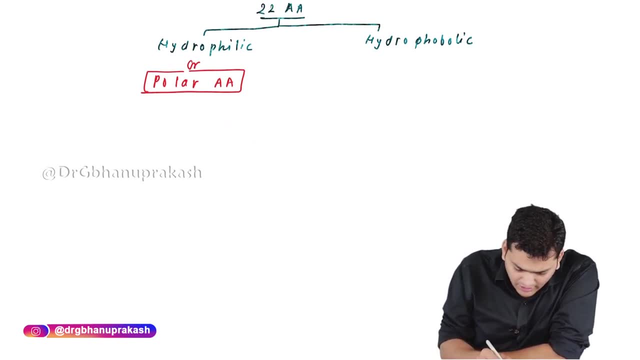 comes to the, the polar amino acid. when it comes to the polar amino acid, how we are going to remember them. see, we are not going to remember the entire list by all the examples of polar amino acid. we will remember by the categories. see how we are going to do. do that if i ask you in a simple way, that 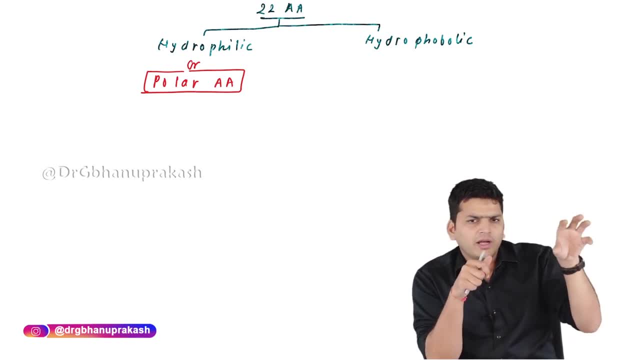 whether the alcohol is water soluble or not means the whiskey, the vodka, they are water soluble or not? yes, you will say yes, they are water soluble. so i can say that wherever there is alcohol, it's going to be water soluble, right? so the alcohol containing amino acid, they are going to be water. 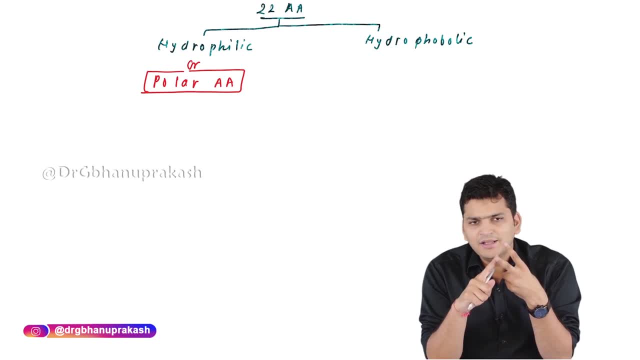 soluble and we have written serine and threonine, serine and threonine, serthero. this is alcohol. serine, threonine, they are water soluble, right? so alcohol containing amino acid water soluble. if i ask you, acid is water soluble or not? yes, acid is water soluble because it contains charge. 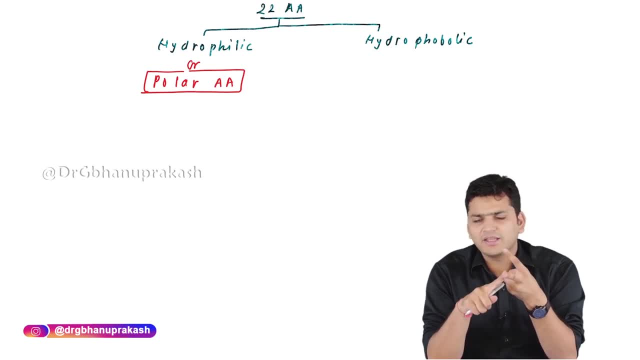 in the same way. basic amino acid. they also contain charge. they are also going to be water soluble and there is a molecule which loves the acid. that is amide. right, so wherever there is amide means there is acid and that is going to be water soluble. so i can. 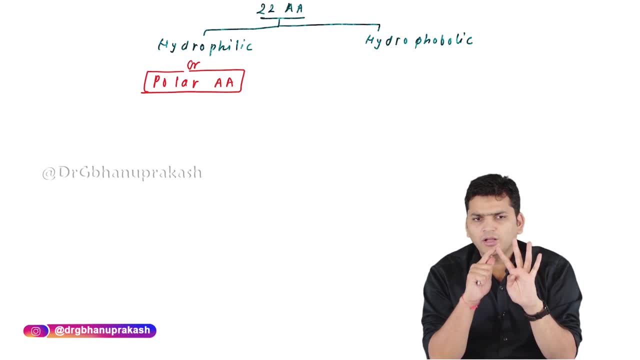 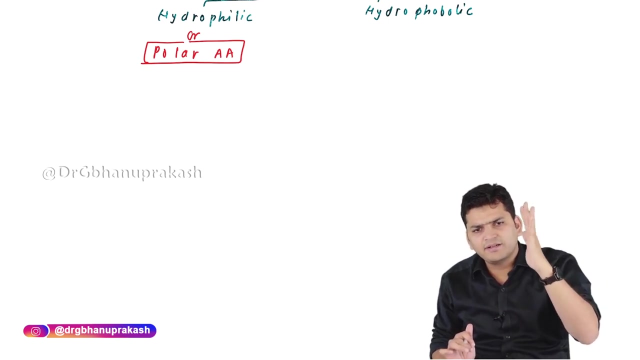 say that there are four categories which are going to be water soluble. one is alcohol, the second is acid, base and amide. these are the water soluble amino acid that we have. so if i write that, the polar amino acid, what are the polar amino acid we have? we have the four sub-categories: alcohol, acid. 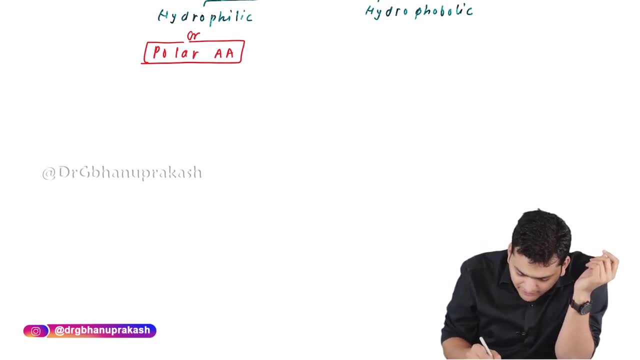 base and amide. this polar amino acid can further be divided into two sub-categories, two sub-categories. that is, Charged Polar Amino Acid. Charged Polar Amino Acid means having a charge or Uncharged Polar. Uncharged Polar Amino Acid. When it comes to the Charged Polar Amino Acid- Charged Polar- 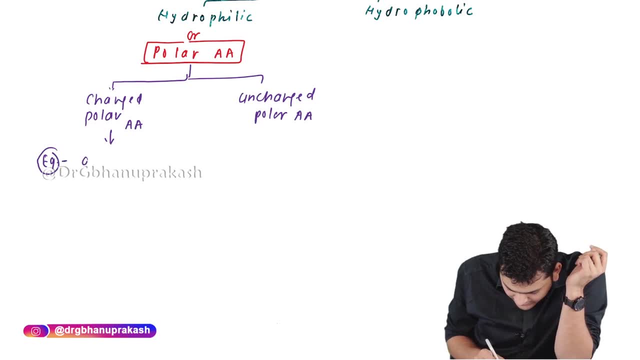 Amino Acid. there are two examples that you have to add: One is the Acidic Amino Acid and the second is the Basic Amino Acid, Because we know that Acid is having negative charge, whereas the Basics are having the positive charge: The Acidic Amino Acid, the examples: 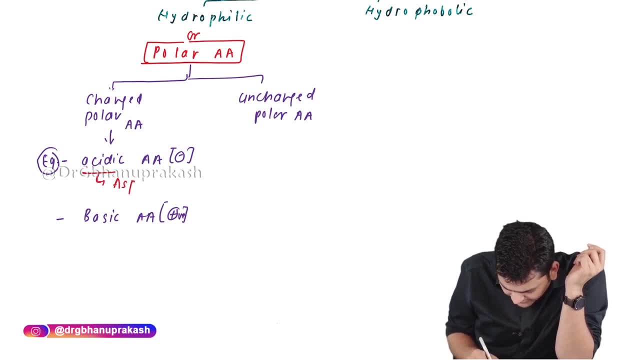 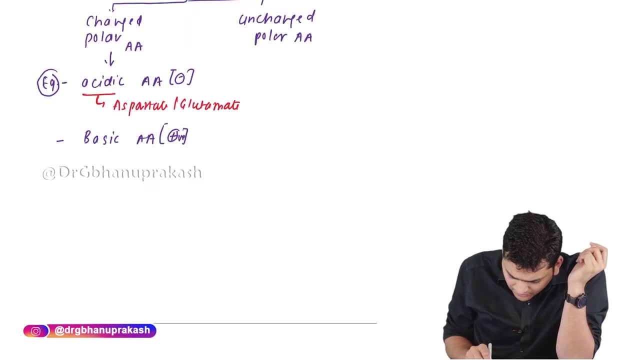 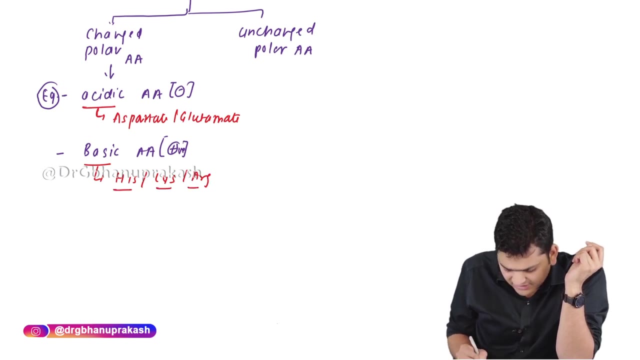 are. we know it's the Aspartate and the Glutamate, That is, the Acidic Amino Acid, The Basic Amino Acid. we have written that the Pneumonic was his last urge. So Histidine, Lysine, Arginine. 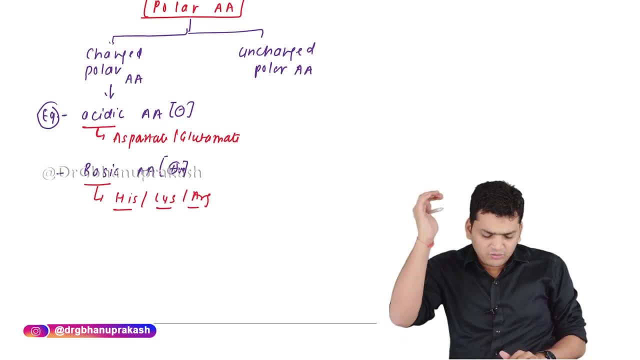 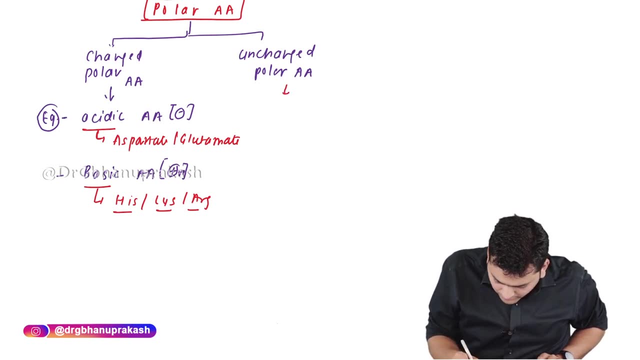 they are the Basic Amino Acid, So Charged Polar. if they say it is going to be Acid and Basic. If they say Uncharged Polar Amino Acid, it is going to be Acid and Basic. If they say Uncharged but Polar, then the examples are going to be: If they say Uncharged but Polar, 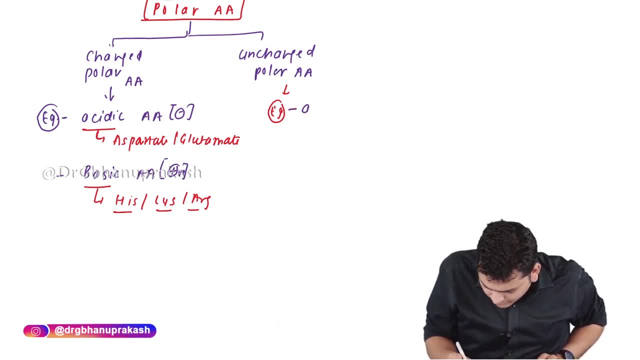 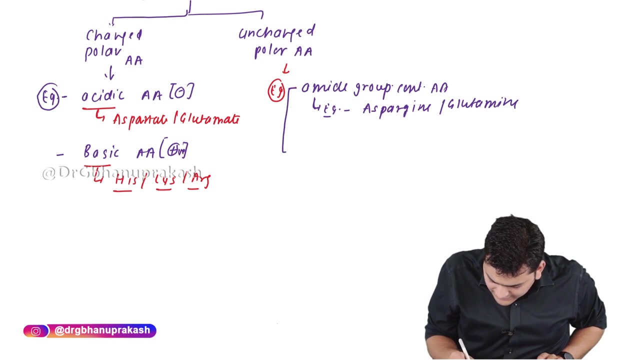 the examples are going to be the Amide Group containing Amino Acid, Amide Group containing Amino Acid, and they are the Asparagine and the Glutamine. Asparagine Glutamine. If they the, then the second category we can say is the alcohol containing amino acid. 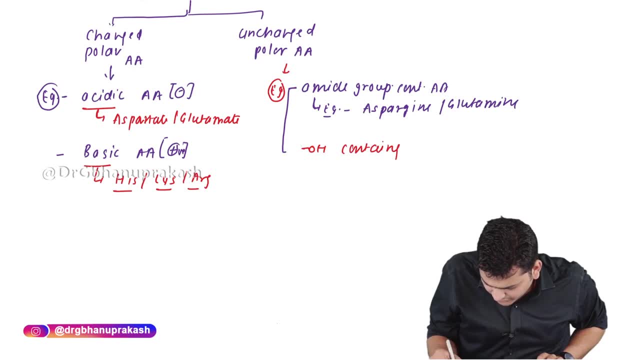 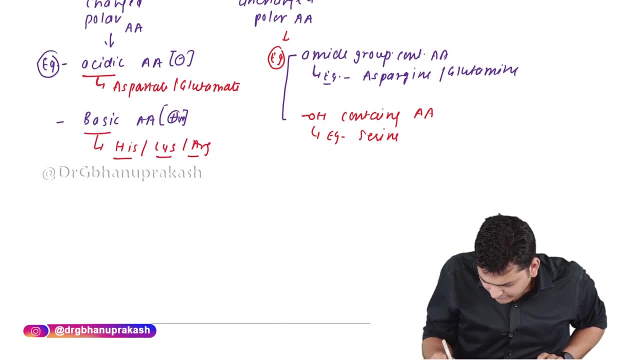 they are also polar amino acid, alcohol containing amino acid. the examples are serine and threonine. if you scroll up the nodes and you see the four subcategory that we have discussed in the classification of amino acid. i told you that alcohol containing, we have three. 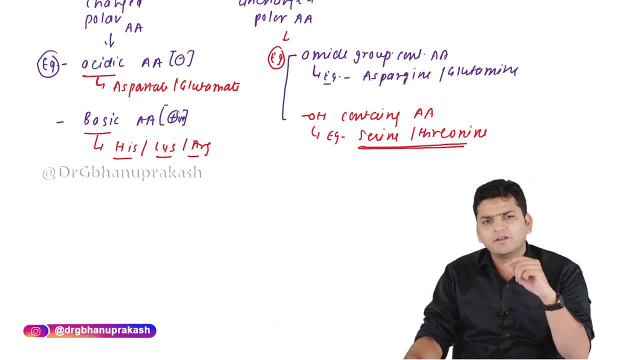 serine, threonine, tyrosine. we have written tyrosine in a separate line. the reason for that is because, despite tyrosine contain hydroxyl group, it is not water soluble. that is why we have written that in a separate line. so these are the polar amino acid. when it comes, 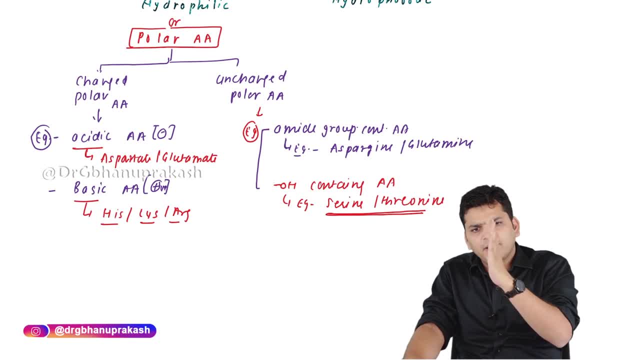 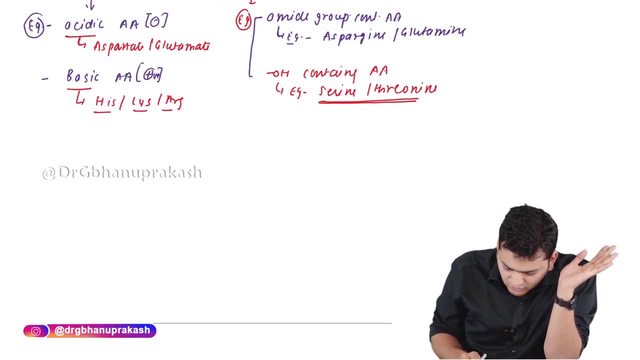 to charged category, acid base. when it comes to uncharged category, the amide and alcohol containing. apart from these four categories. apart from these four categories, there are two more amino acid which are water soluble. their entire category is not water soluble, but they are indivisible. 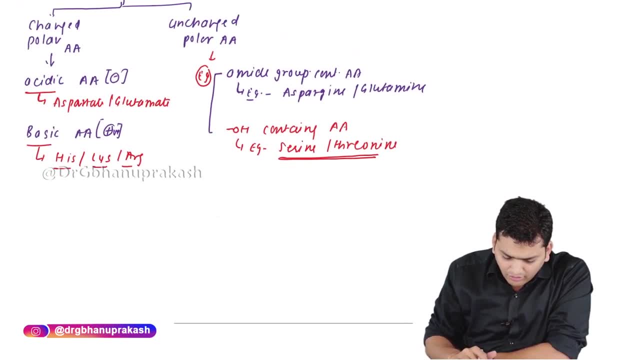 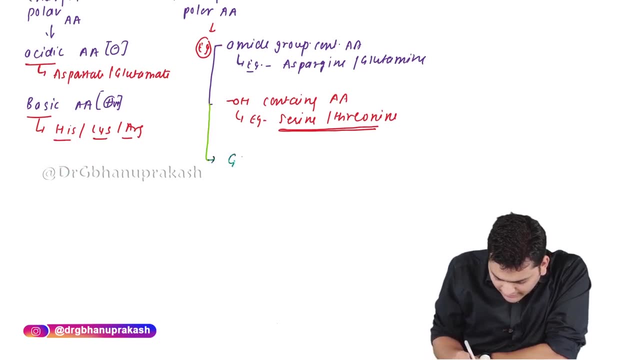 they are water soluble, so they will come under the category of uncharged polar. apart from these, we have two more amino acid which are water soluble, and that is glycine and cysteine. glycine is a simple amino acid and the cysteine is a sulfur containing amino 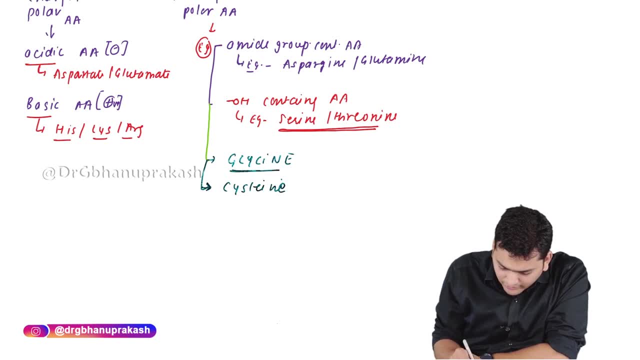 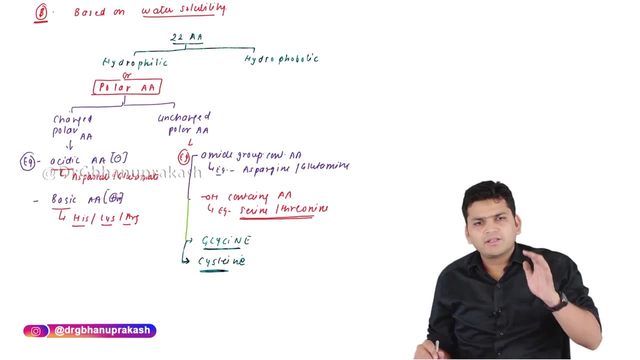 acid. their entire category is not water soluble, but these two are water soluble. these two are water soluble. so this is the complete classification of the, the hydrophilic amino acid. now let's say what are the four categories: acid, base amide and alcohol. apart from these, 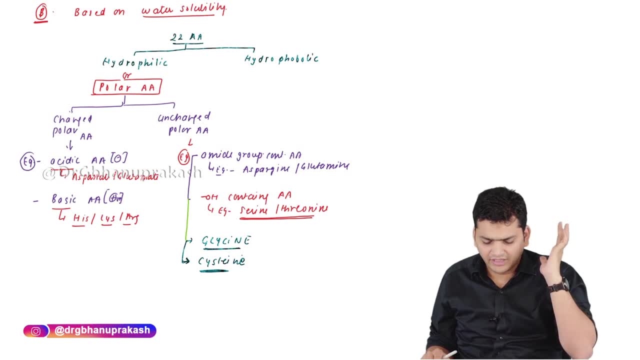 four, which are two individual amino acid which are water soluble: glycine and cysteine. remaining- all remaining- all are hydrophobic. so when it comes to hydrophobic, i can say: remaining- all remaining- all are hydrophobic. so this is the classification of amino acid based on: 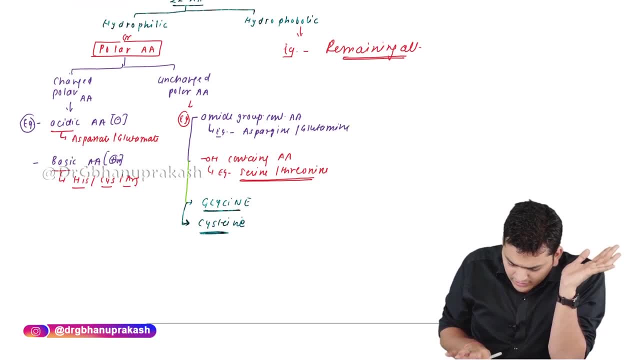 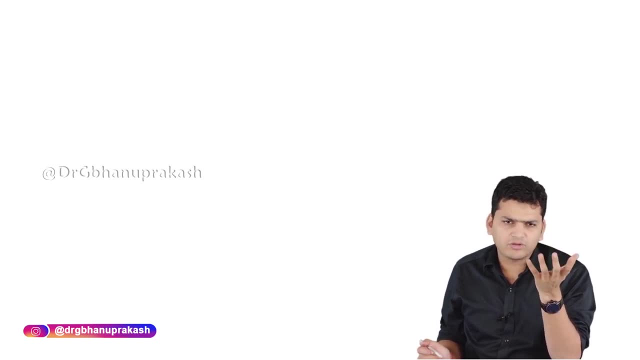 water solubility, whether they are water soluble or not. now here are some controversial questions, so how to answer them? there is some controversial part that is there in this hydrophobic water solubility, so i will try to give you a best idea that what is the best possible choice. 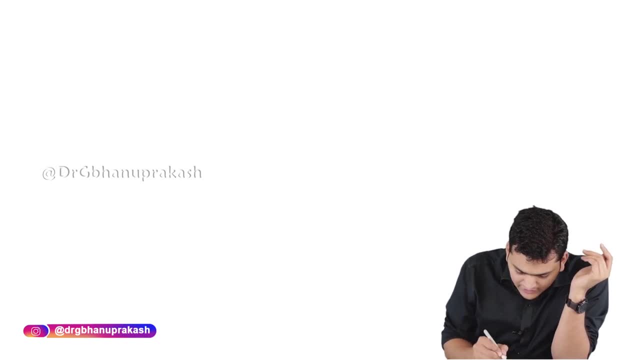 that you can select in a multiple choice question. if we see that which is the most water soluble, if we see the most hydrophilic amino acid, the most hydrophilic amino acid that we have is arginine, arginine- arginine- that is the basic amino acid, is most hydrophilic. 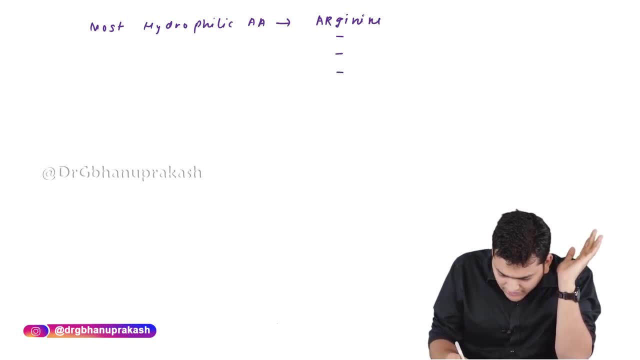 the hydrophilic category. there are some other examples. we have discuss them right. so when you reach to the bottom, the least water soluble among the water soluble category means having the the least characteristic of having water solubility among the water soluble is glycine. 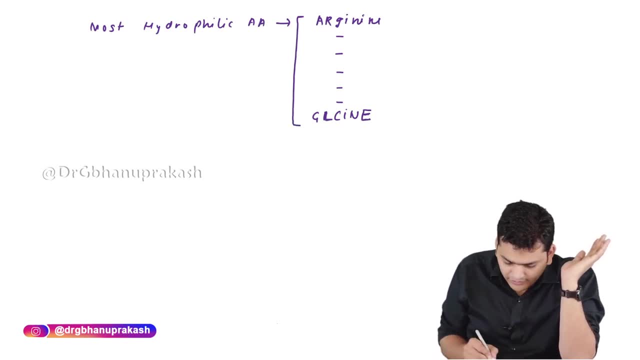 so these are the hydrophilic amino acid that we have. when it comes to the hydrophobic, when it comes to the hydrophobic, the least hydrophobic among the hydrophobic category is tyrosine. then there are several examples and then we'll reach all the way, bottom that 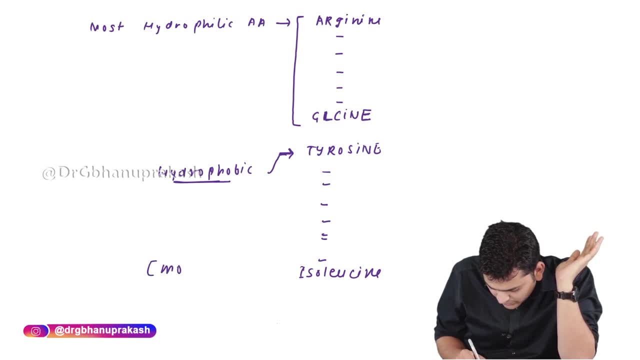 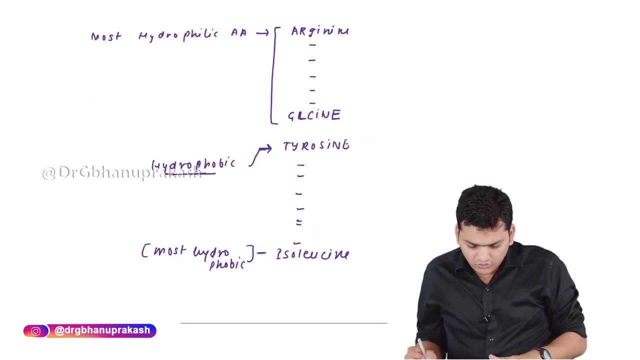 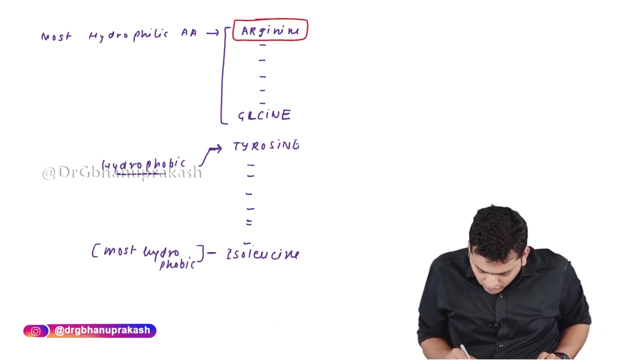 is isoleucine, which is the most most hydrophobic. most hydrophobic is isoleucine. so this is the order. this is the order that arginine is the most water soluble, the least water soluble is isoleucine, and somewhere in between we. 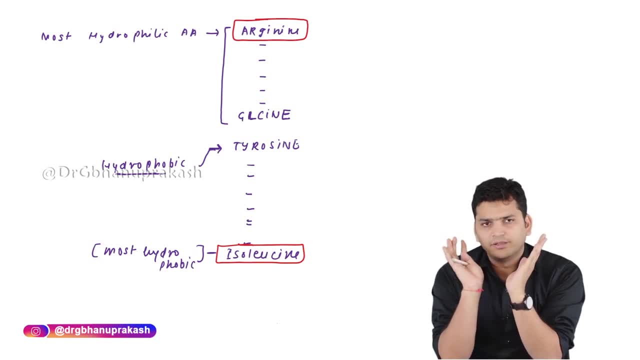 are going to have the glycine and tyrosine on the borderline where they are going to meet right. so glycine is the least water soluble in the water soluble category. if you take all the water soluble which is having least water solubility among the, that four is going to be glycine. and if you see, 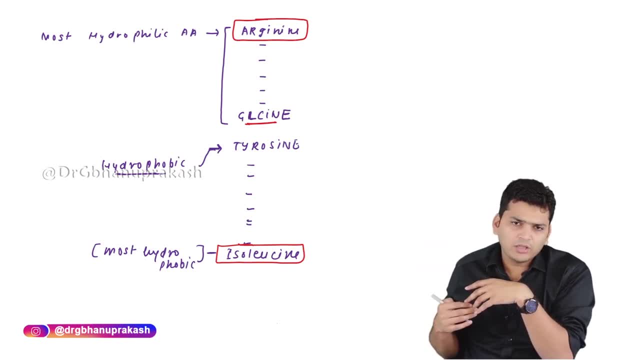 that the, in among all the hydrophobic, in among all the hydrophobic, which is having the maximum potential to be a water hydrophilic amino acid? the answer will be tyrosine. that this tyrosine can go to the upper category also. so this is the gray area. this is the gray area. 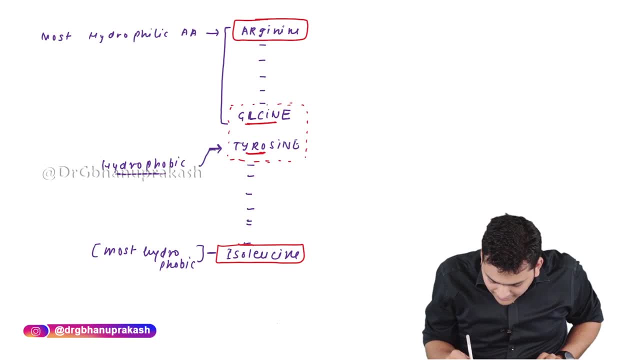 so when the question will be asked from this particular part, then you have to select the answer based on the given option. based on the given option, say, for example, if i ask you that all of the following are water soluble, except if the question language is like that: 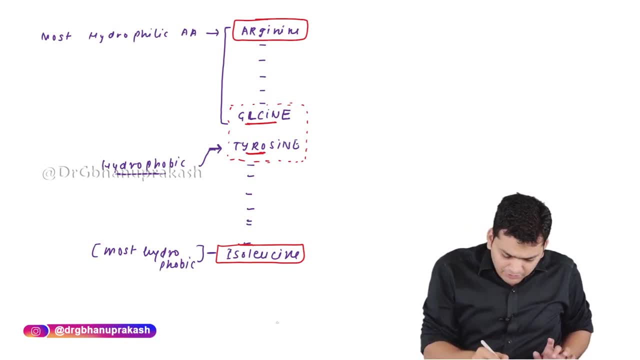 all of the following are water soluble except, and the three options are: arginine, glycine, tyrosine and- let's say, someone is from here- or maybe isoleucine, right? so which one you are going to choose? you are going to choose this one. you are going to choose this one, right? if? 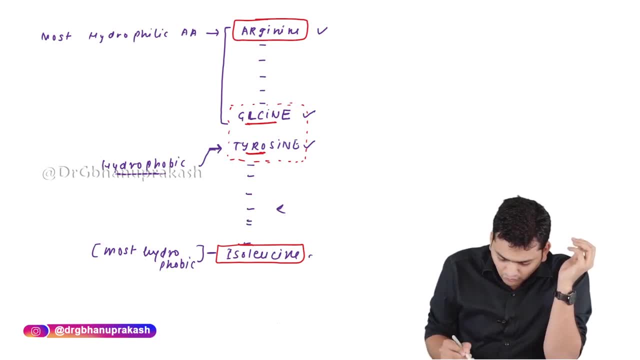 they have given three options. if they have given three options from, like that see here, the first option is arginine, then one option is from here, let's say serine, the third option is glycine and the fourth option is tyrosine. if these are the four option and they're asking that, 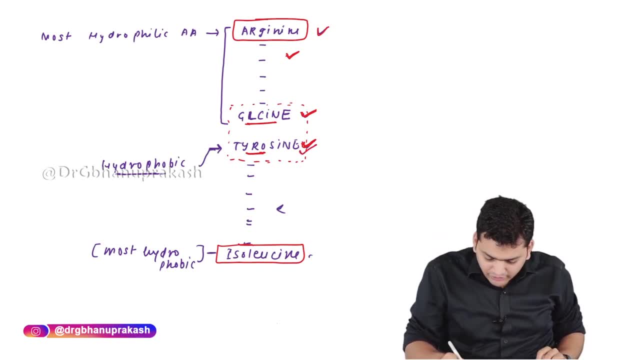 which is water insoluble, then the- the answer is very straightforward- is going to be tyrosine, right? so, depending on option, you have to choose from this particular gray area. so this is one controversial part and this is how you have to find the answer in that controversial part. 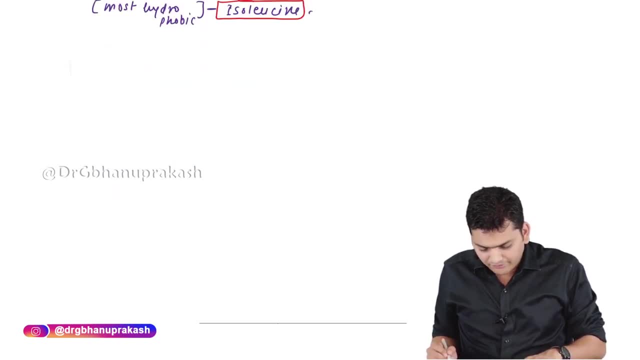 this is the second classification that is based on the water solubility, the. the third type of classification that we are going to discuss is based on the metabolism, based on metabolism of amino acid. when you do the metabolism, what you are going to notice? that when you metabolize these various 22 types of amino acid, you are going to notice that we can get several types of metabolite, and one of them is ketone body. if you generate ketone body from the amino acid, you will get the amount of oxytocin that you are taking and that is going to be the amount of ketone that you are ingesting, that you are taking. so this is the point, which means whenever acid metabolize. such amino acid are called as ketogenic amino acid. they are called as ketogenic amino acid. there are some amino acid which can generate glucose on their metabolism. they are referred as glucogenic amino acid. they are referred as glucogenic amino acid. so we have ketogenic amino acid. we have 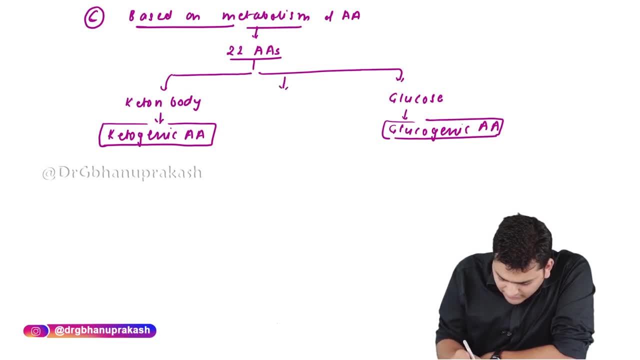 glucogenic amino acid. there are some amino acid which can generate ketone body and glucose, both depending whatever is the demand of the body. either body requires ketone body, they will generate ketone, then the body requires glucose, they will make glucose. so they are called as keto plus glucogenic. 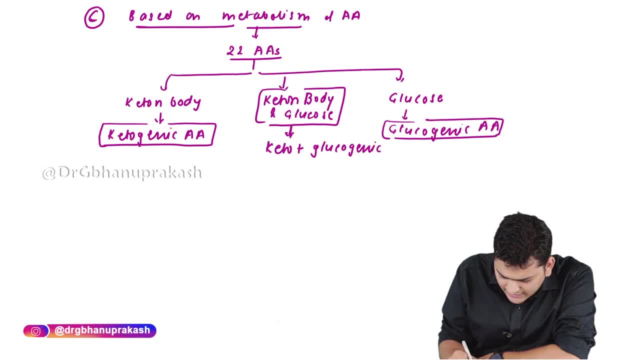 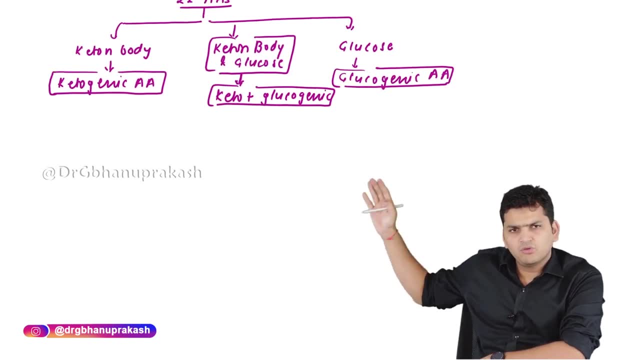 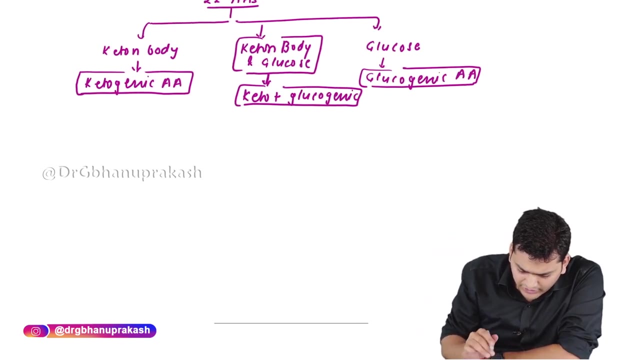 keto plus glucogenic. so I can say that there are three subcategories based on the metabolism of amino acid. it can be ketogenic, keto plus gluco and the glucogenic. keto, keto plus gluco and the glucogenic. when it comes to the example of ketogenic amino acid, there are two examples to be remembered. one is: 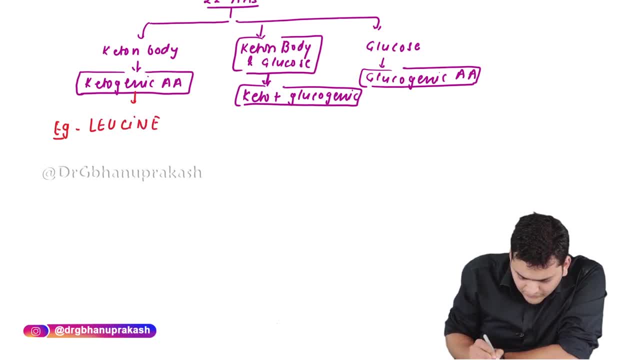 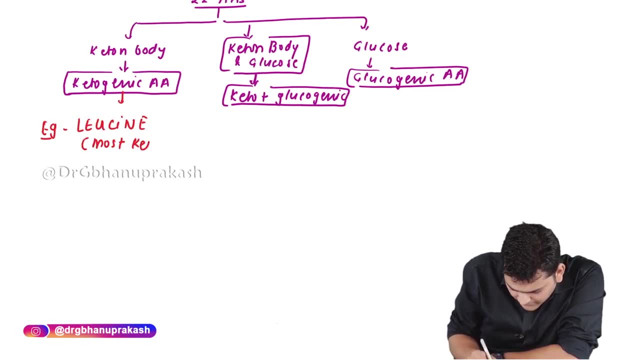 leucine. leucine is the most ketogenic amino acid. among all the ketogenic is the most ketogenic. most ketogenic is leucine. then the second we can add is lysine, which is also predominantly ketogenic. so leucine and lysine, they are ketogenic, but among 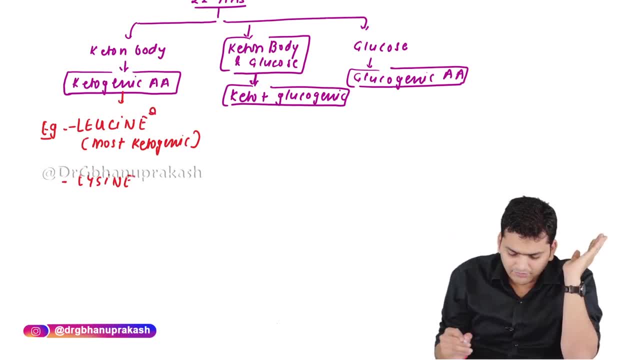 these two. if you have to select one which is most ketogenic, the answer is leucine. the answer is leucine when it comes to keto plus glucogenic. keto plus glucogenic. the examples are tryptophan, phenylalanine, tyrosine and isoleucine. these are the four amino acid which are keto plus glucogenic means they can make ketones as well as glucose, depending on the demand. the third category is the glucogenic amino acid. so I can say, in the example of glucogenic amino acid is the. remaining all the amino acid are glucogenic. remaining all the 16 amino acid are glucogenic. but if they ask that which is most glucogenic among the remaining ones, which is the the most glucogenic is alanine, most glucogenic. is alanine most glucogenic? the answer is alanine. so most ketogenic leucine, most glucogenic is alanine. is alanine. so this is the second classification. that is, the third classification that is based on the metabolism. that is based on the metabolism: amino acid, ketogenic, keto plus glucoa and the glucogenic. the fourth classification of amino acids, the fourth classification of amino acid that is based on the nutritional requirement: classification based on nutritional. 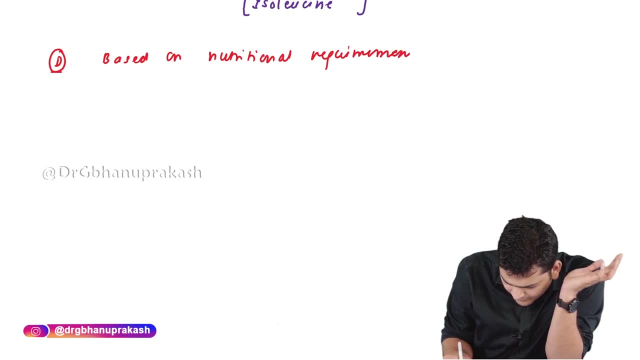 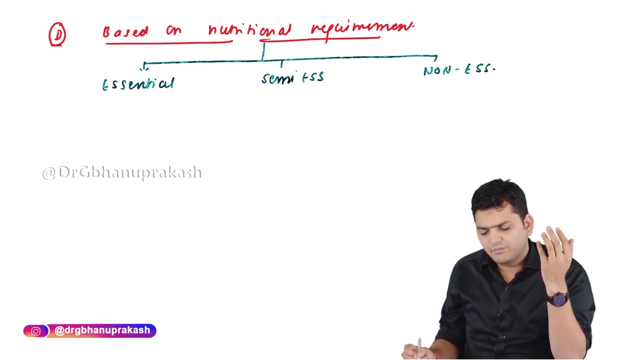 requirement classification: amino acid based on nutrition requirement, The sub category you may have heard about specifically about them earlier. also the based on nutritional requirement. the amino acid are classified into three categories. classified into three categories: the essential, semi-essential and the non-essential. essential, semi-essential and non-essential. these are the. the amino 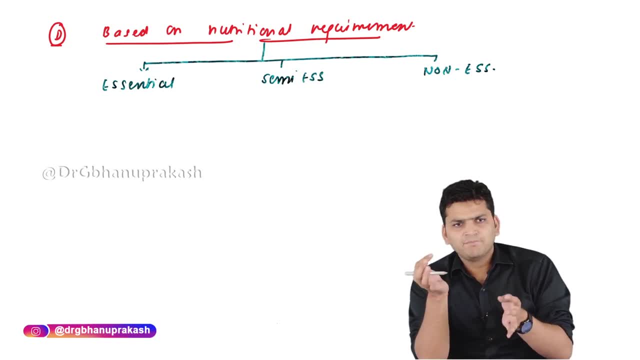 acid category is based on the nutritional requirement. what is the meaning of essential? essential means that these are the amino acid. you have to take them in your diet. the body cannot synthesize them endogenously. they are called as essential. non-essential means whether you eat in your diet or 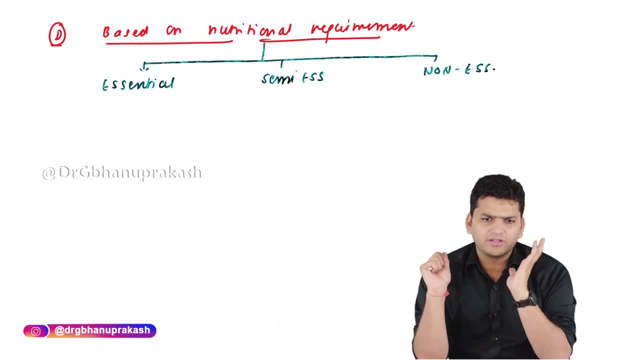 not. the body is going to synthesize them endogenously. they are non-essential. whether you take them in your diet or not, the body will take care of that. that are non-essential. now, the semi-essential amino acid are those amino acid which are required during the time of growth means when we were in the pediatric age. 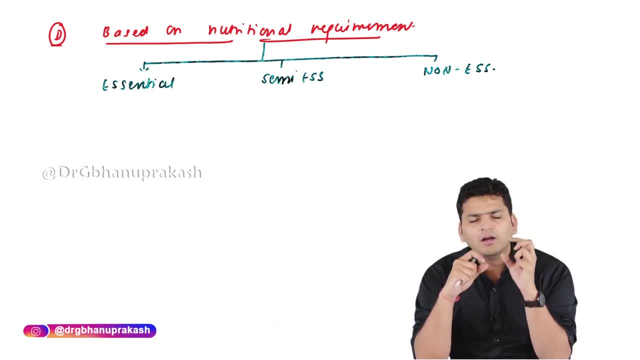 group during the time of growth, that where these amino acids are required, they are come under the category of semi-essential. so there are three categories: essential, semi-essential and non-essential. so let's see the examples of essential amino acid. when it comes to the essential amino, 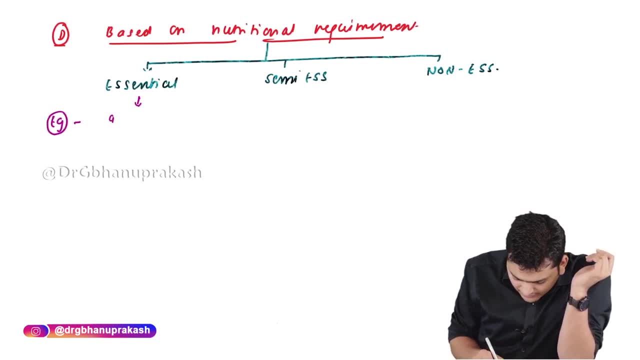 acid. first, we need to remember that there are nine amino acid. there are nine amino acid which are essential. we have nine essential amino acid out of 22 we have. 9 are essential to the pneumonic, for which are the essential amino acid we have the pneumonic that we are. 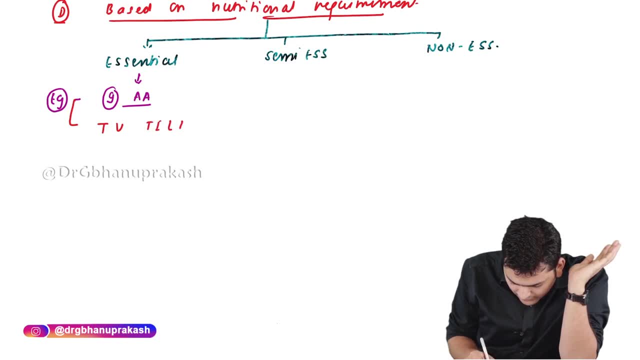 going to use. is TV till 9 pm H. TV till 9 pm H. TV till 9 pm H is the example for the 9 essential amino acid. for example, if I say isoleucine, is it essential or not? you? 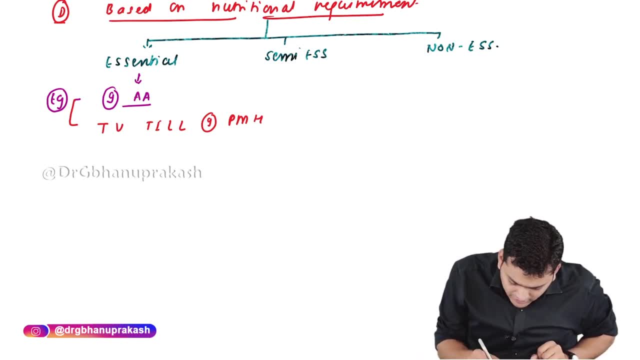 will see, the initial isoleucine is I and you will search whether the I is there in the pneumonic or not. yes, I is there. so you will say it is essential. in the same way, what they do is they will try to confuse you between three options. between three options, say, if 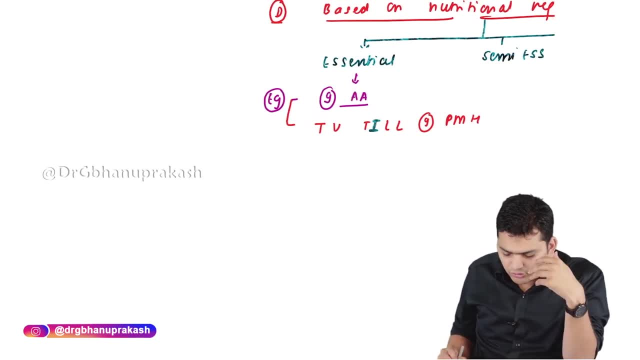 I see the amino acid, the set of 22 amino acid. what I am going to notice? that there are three amino acid that starts with the letter T. if I ask you that which amino acid starts with the letter T, you will say tryptophan, tryptophan. yes, rightly. 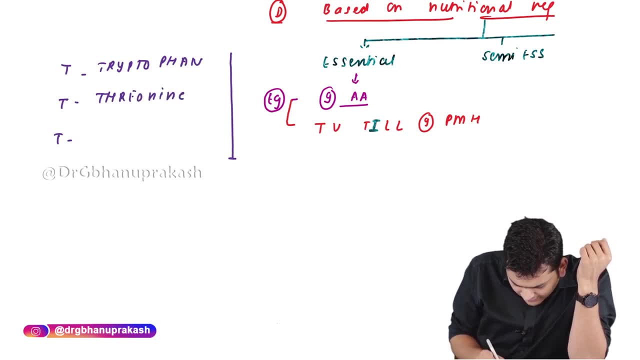 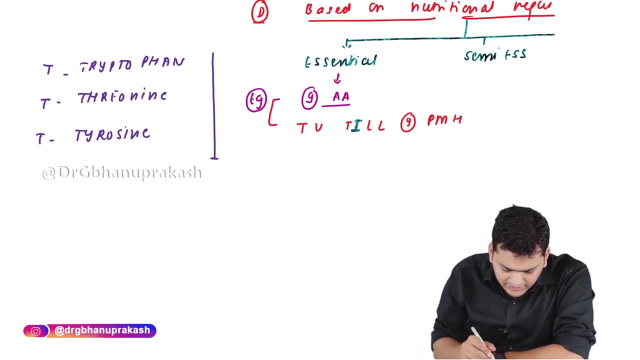 is threonine and the tyrosine. these are the three amino acid, amino acid that starts with the letter T. now, if they ask that, which are the essential amino acid, and these are the option, these are the option. so you will use the pneumonic TV till 9 pm. H, if you see. 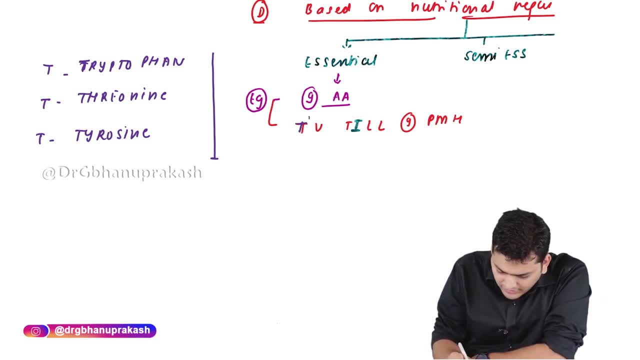 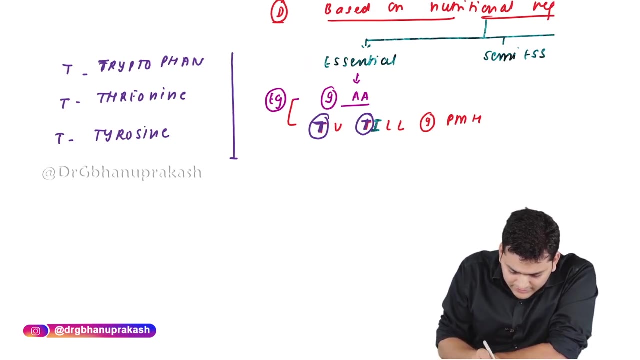 the pneumonic. how many T's are there? there is one T, TV till. so again one more T, so there are two T. but how many amino acid starts with the letter T? tryptophan, see threonine and the tyrosine. so this tyrosine starts with the letter T, it is non-essential. it is non-essential. 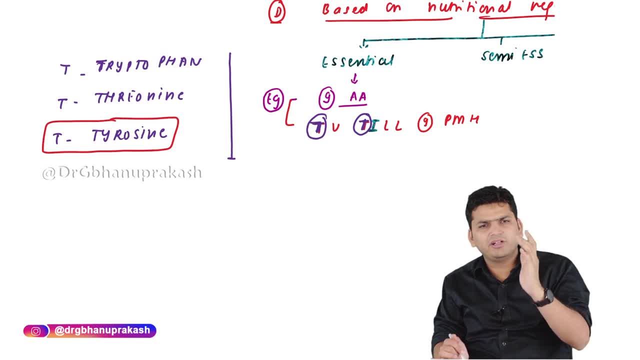 so we need to remember the. the examiner knows that you are going to use the pneumonic TV till 9 pm H, so they will try to confuse you between tryptophan, threonine and the tyrosine. so we should know that tyrosine is a non-essential amino acid if you are using this pneumonic. 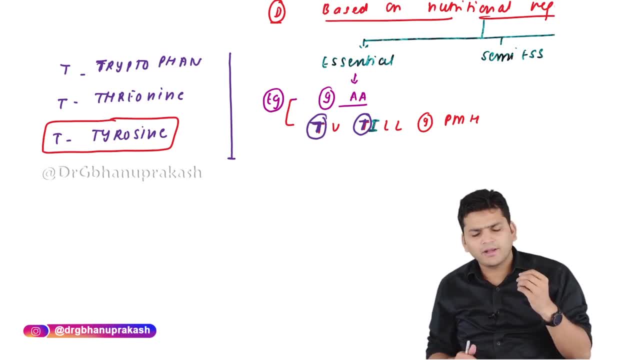 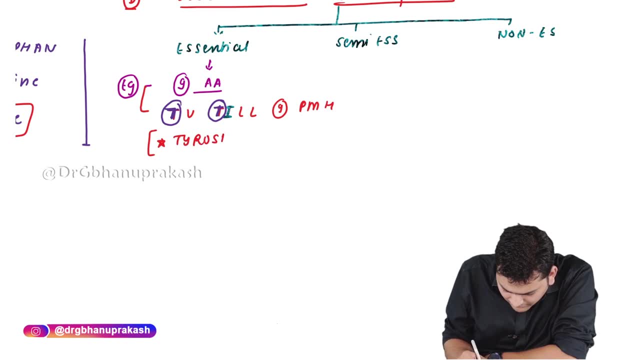 the thing that has always kept, always have to be kept in mind, is that the tyrosine is non-essential. so I am writing this statement here is: tyrosine is the non-essential amino. tyrosine is non-essential. If you remember these three things- 9 essential- we have TV. 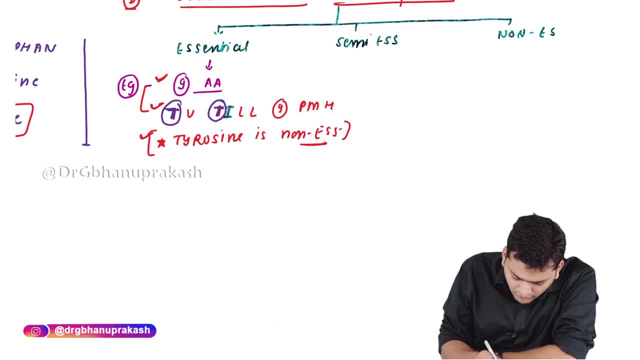 till 9 PMH. tyrosine is non-essential. All the MCQs are going to be correct when it comes to the category of essential amino acid, right? If you want to write all the 9 names, all the 9 names, what are the TV till 9 PMH. what are the 9 names are? you can see in the list. 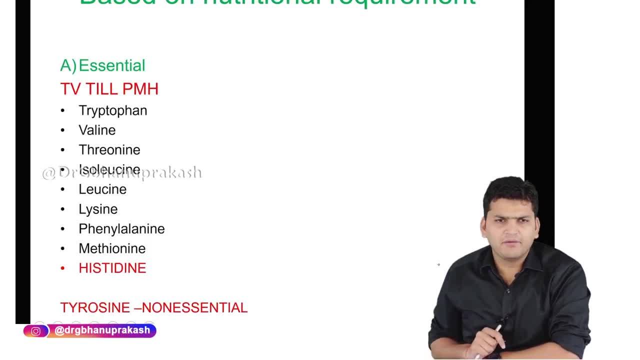 here. These are the 9 essential amino acids we have. These are the 9 essential amino acids, So you can see it's the tryptophan, valine, threonine, isoleucine, leucine, lysine, phenylalanine. 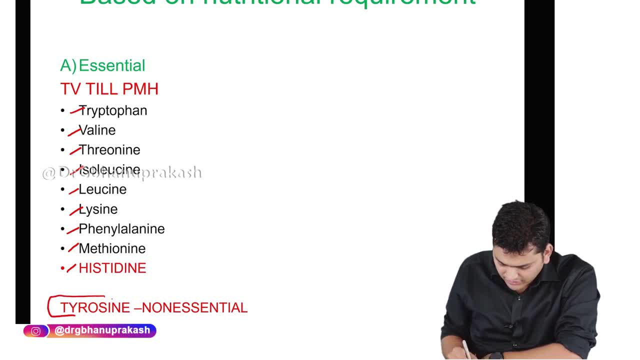 methionine and histidine. Tyrosine is non-essential, Tyrosine is non-essential right. So in some books, in some books you might find histidine is not written in essential. In some books it might be written in semi-essential category, semi-essential category. So that is again. 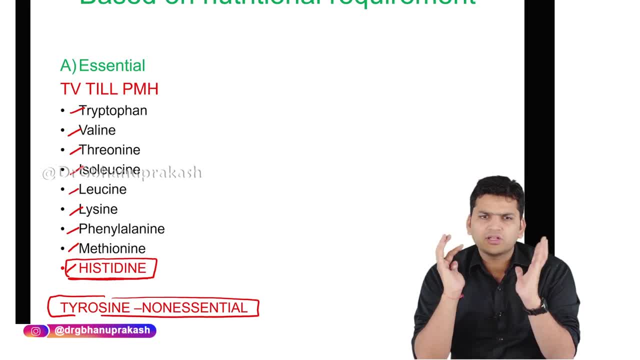 we can say a controversial part. I will tell you how to solve such MCQ also. Right, So the essential category, the essential category, initially we will, we will have this concept that we will retain the histidine in the essential category only and the pneumonic. 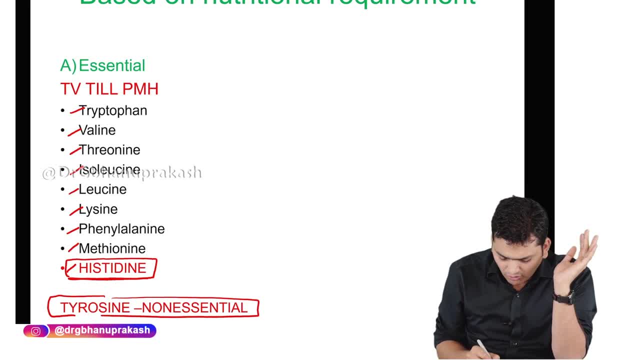 is going to be TV till 9 PMH. Tyrosine. non-essential. Histidine is a controversial part. Some books says it may consider as semi-essential. right, When we see the negative nitrogen balance then we find that histidine is not the semi-essential. it is the essential amino acid, But still. 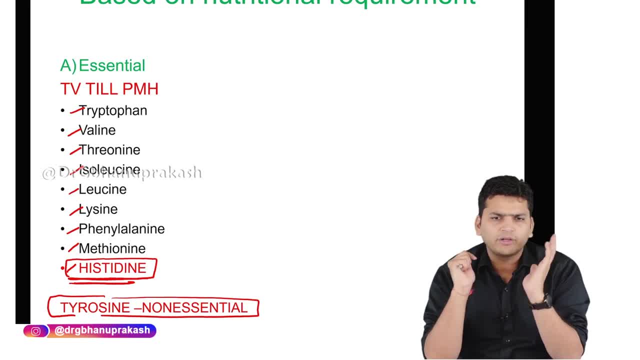 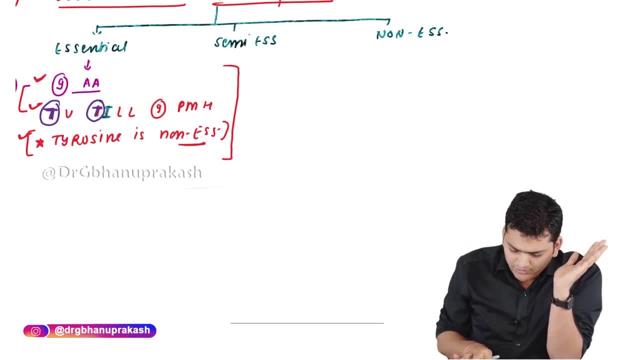 in some books it is written as semi-essential, So we will always have to keep that thought in our mind while solving the MCQ. So these are the essential amino acid that we have. Now coming to the semi-essential category. in the semi-essential category, the only example- 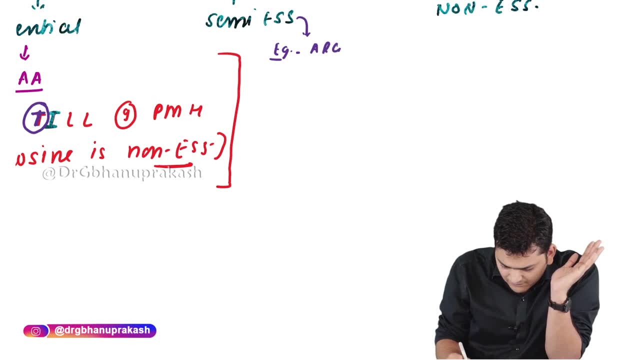 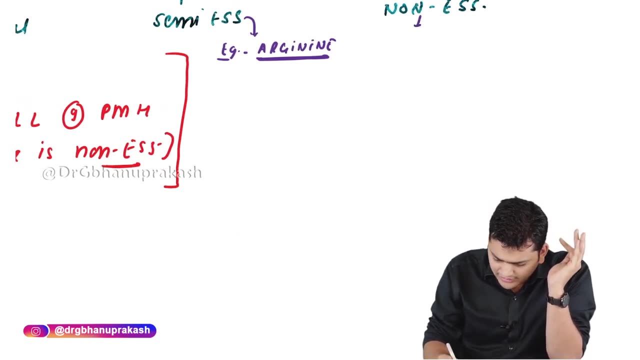 that we have to remember in mind is arginine. The only example is arginine that we have to keep in mind. The third category is non-essential. The examples are: remaining all the 12 amino acid remaining all 12 amino acid are going to be non-essential. 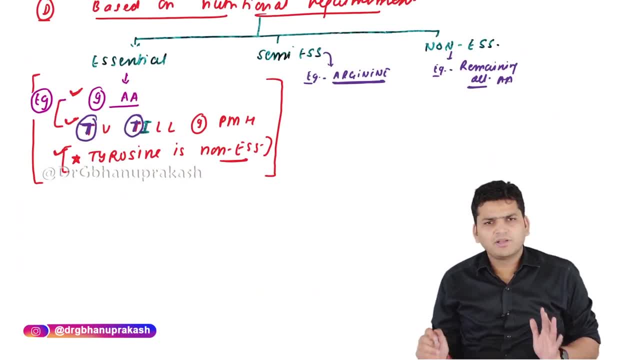 We have the essential, semi-essential, non-essential. There is a controversial part regarding the histidine Histidine. in some books it is essential, In some books it is semi-essential. So when you are solving the MCQ and they are asking: 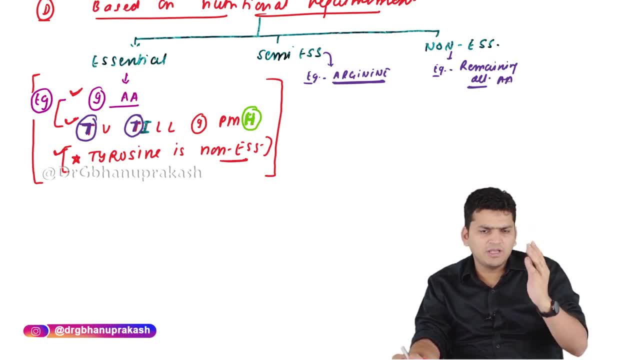 which of the following is semi-essential? and in that question, arginine is not given in the choice. Instead of arginine, histidine are going in the choice. Then you will select histidine and semi-essential, right. so it all depends on the options that are given to you. 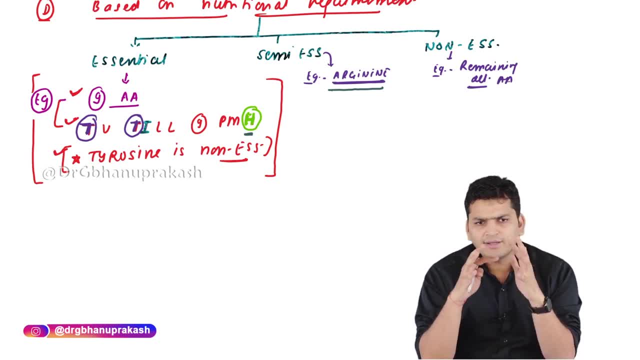 depending on that, we have to find the best option. so, as i told you, as example, that if they say which of the following is semi-essential- arginine is not in the option, then the second best answer is histidine, right? this is the the fourth classification that is based on the nutritional requirement. 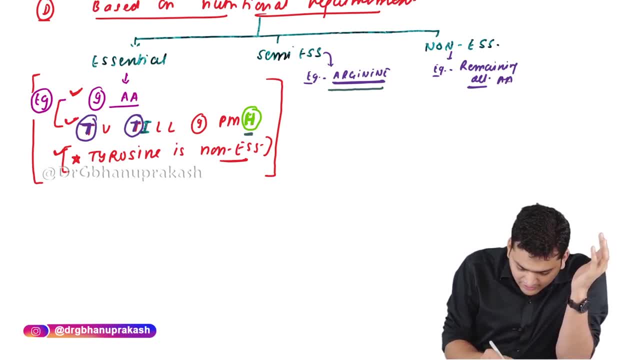 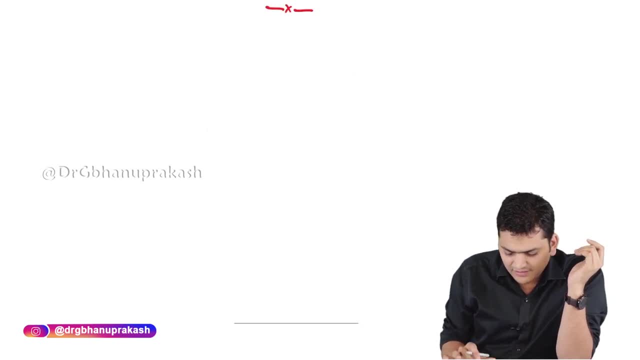 the next thing is there are- this is the. this is the fourth category of classification. that is completed. then there is a special property of amino acid, that some amino acid have a specific order or a specific smell. right, these are called as aromatic amino acid. so this is a ectopic variety. 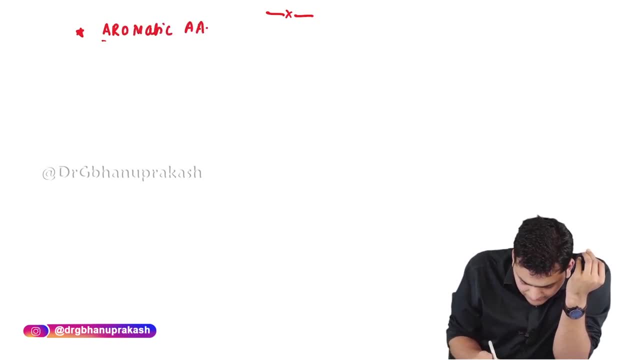 we can say it's the aromatic amino acid means they have a peculiar order or a peculiar smell. they are called as aromatic amino acid. so what is important is to remember is the example. what are the example of aromatic amino acid we have you. so to remember the aromatic amino acid, i will just tell you a simple. 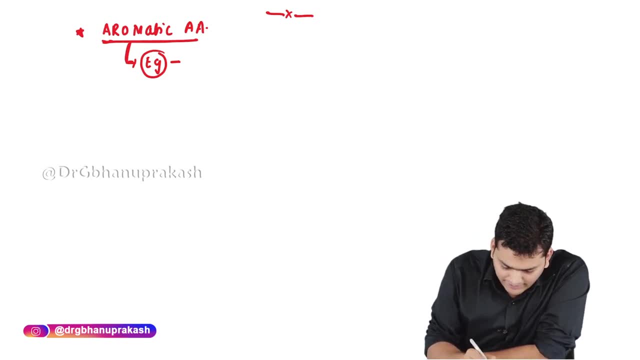 uh, mnemonic, how to remember the aromatic amino acid, for example? let's say, right now we are having this class in a closed environment. let's say, all the clothes, all the doors, all the windows are closed. now what i do is, uh, i bring a rubber tire in this classroom and i burn the tire. i burn the. 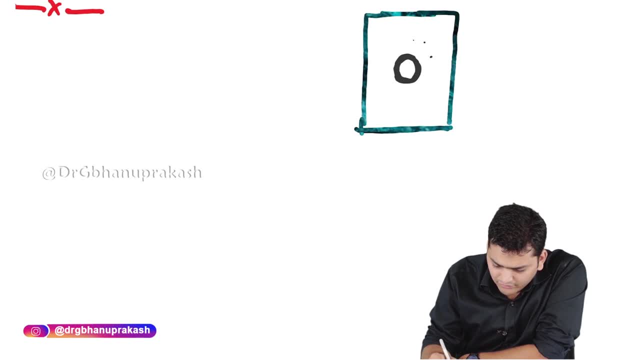 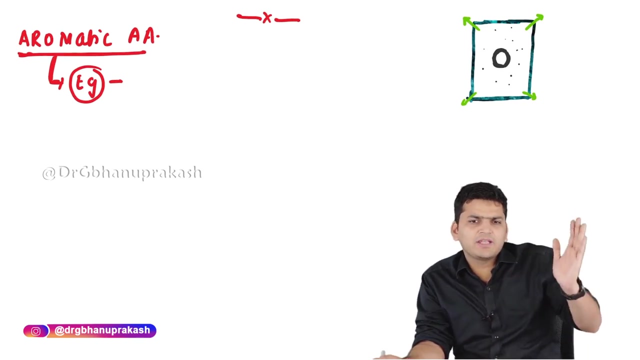 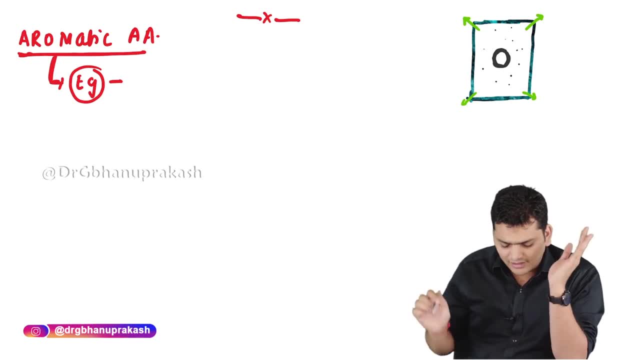 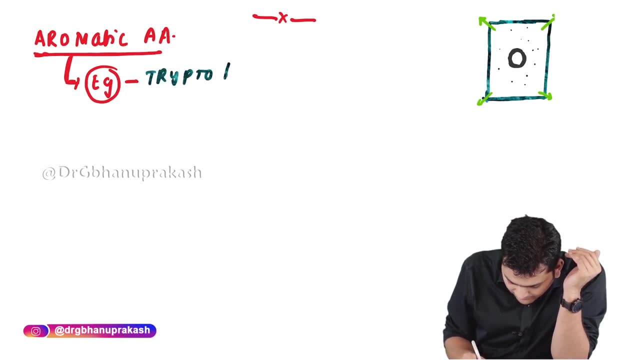 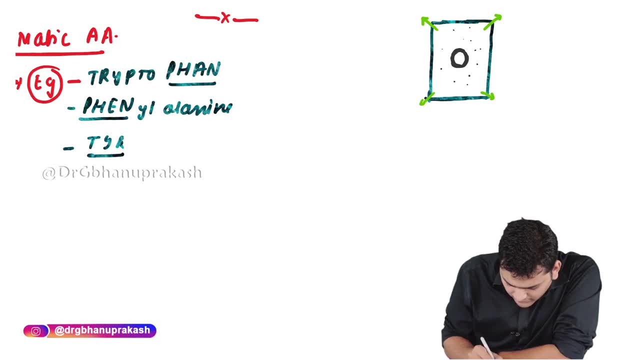 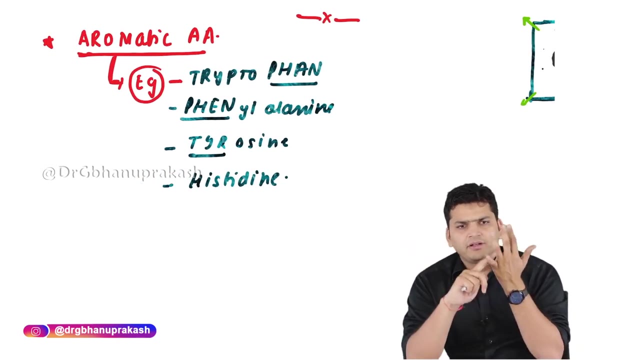 so tyrosine is aromatic amino acid apart from these. the fourth one is histidine. histidine, that is also aromatic. so the first thing you can easily remember by the new money fan in the name. what is the smell this time? tryptophan, phenylalanine, tyrosine. the fourth, 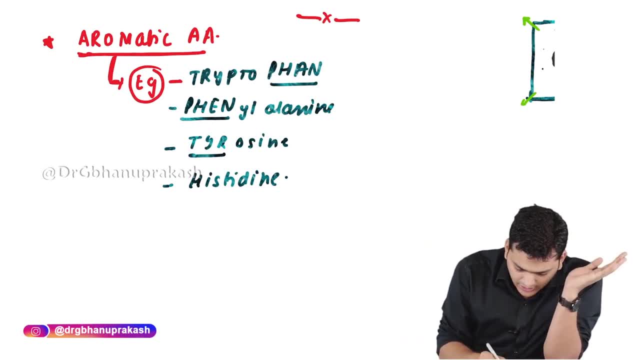 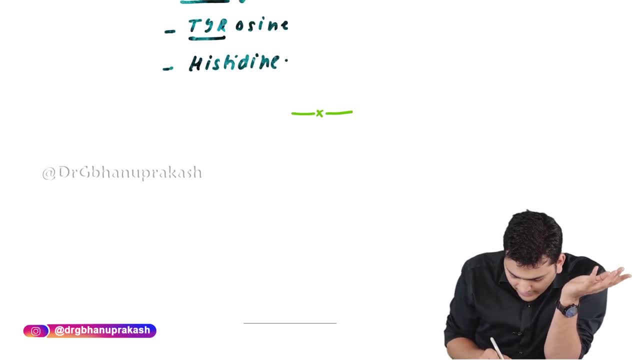 one is histidine. these are the aromatic amino acid we have, so this is a ectopic variety of amino acid. there is one more ectopic variety of amino acid and that is referred as derived amino acid. derived amino acid. let's understand what is the meaning of derived amino acid. 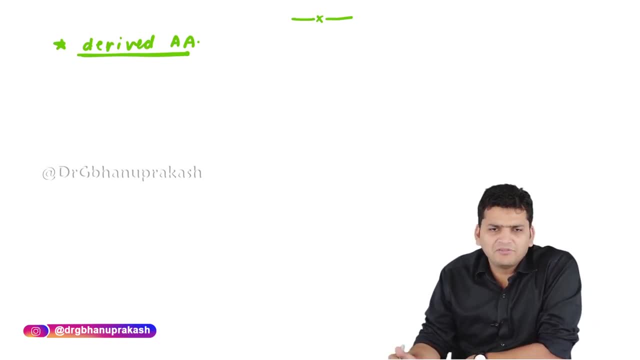 so to understand the definition of derived amino acid, i will just use a simple concept that see the most of the amino acid, most of the amino acid, say, for example, methionine. methionine is amino acid. it is represented by a codon. every amino acid will be represented by your codon. the codon for methionine is a, u, g. 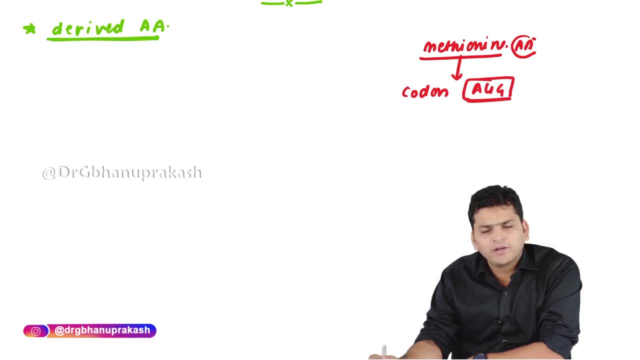 we'll discuss that in detail when we will discuss genetic code, right? but for now, every amino acid is represented by a codon and for methionine the codon is a, u, g, but there are some amino acid which cannot be represented by a codon. if amino acid cannot be represented by your codon, that is. called as derived amino acid. that comes under the category of derived amino acid. so what is derived amino acid? amino acid which cannot be represented, which cannot be represented by codon, that is referred as the derived amino acid. usually the amino acid is represented by a codon, but if amino acid cannot be represented by a codon, it's called as derived amino acid. 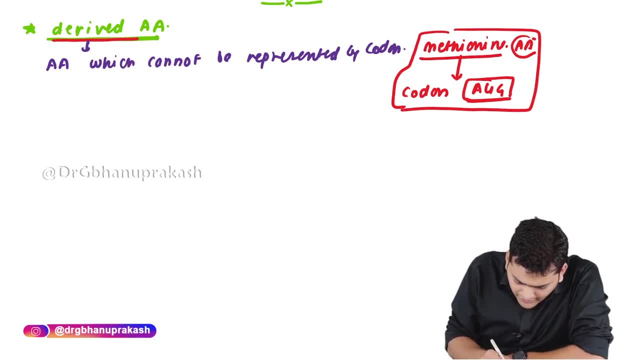 so what is important is the example, the example of derived amino acid, the example of the amino acid here we're looking at. the first example is hydroxy proline. hydroxy proline- this is found in collagen, found in collagen pro tee. collagen is a protein. the hydrogen program is found in collagen. 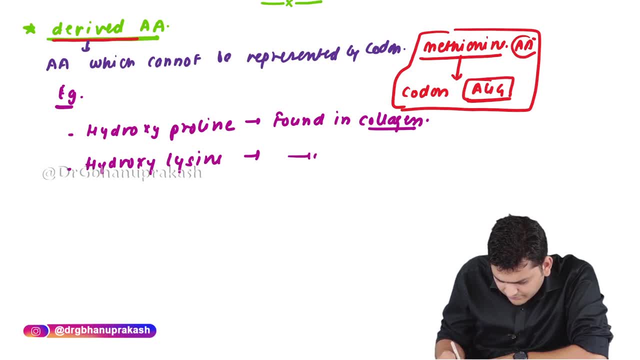 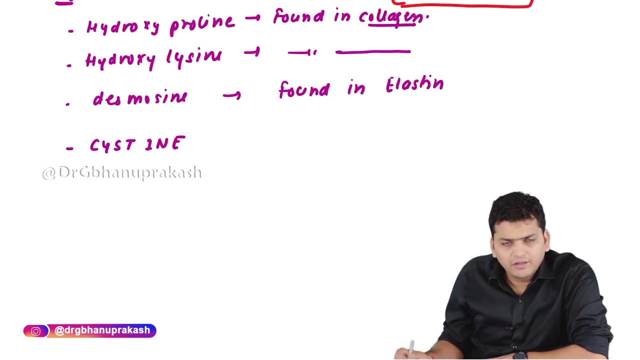 then is the hydroxy lison, hydroxy lisen acid, found in collagen. Then the next example is desmosine. It is found in elastine. Then the fourth example is cysteine. The cysteine molecule should not be confused with cysteine. Cysteine is a sulfur containing amino acid. So what is cysteine and what is cysteine? What is the difference between them? So what I do is: we know that cysteine is a sulfur containing amino acid. What I do is I take two molecules of cysteine. Let's say this is the first molecule. 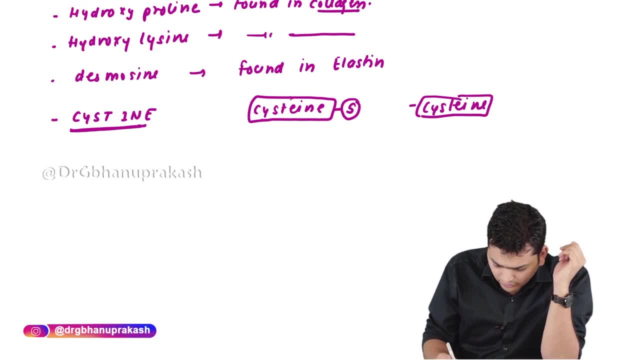 and this is the second molecule of cysteine. I take two molecules of cysteine. I join these two cysteine molecule between by these two sulfur molecules. So this is the bond that i am going to have is the disulfide bond. disulfide bond. so if you take two cysteine, molecule join via the disulfide bond, this entire unit that you have got is going to be referred as cysteine. this entire unit that you got is referred as cysteine, right? so what they ask is: the cysteine is found where? cysteine is found in those molecule which contains disulfide bond, wherever we requires. disulfide bond. we will place cysteine molecules because we know that cysteine is having disulfide bond. so the example where it is found cysteine is found in insulin. insulin protein contains a disulfide bond, so that we require cysteine. one more example that i can add is immunoglobulin. that is, antibodies. that also requires cysteine molecule. insulin and immunoglobulin. they require the cysteine molecule. the other examples of the derived amino acid. so we have discussed four examples of derived amino acid: hydroxyproline, hydroxylysine, desmosine and 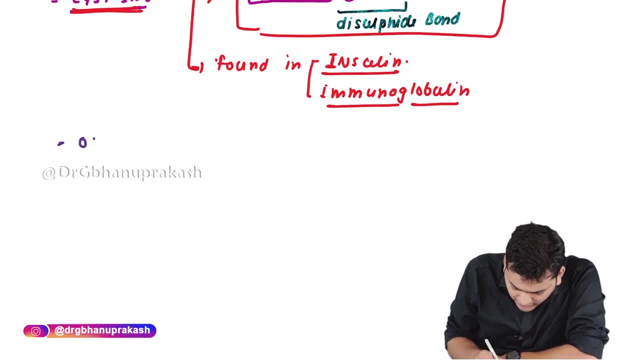 cysteine. few more examples that i can add is ornithine citrulline: ornithine citrulline. these are the other examples of the derived category, right? so there are many others also, but at least you should remember these six. at least you should. remember these six. these are the six amino acid which are, uh, the derived amino acid. so this is the complete classification of amino acid. this is complete classification. we have divided the amino acid base mainly in four subcategories: based on r group, then based on the- the water solubility. then we have discussed about the. based on the- their metabolism, keto. 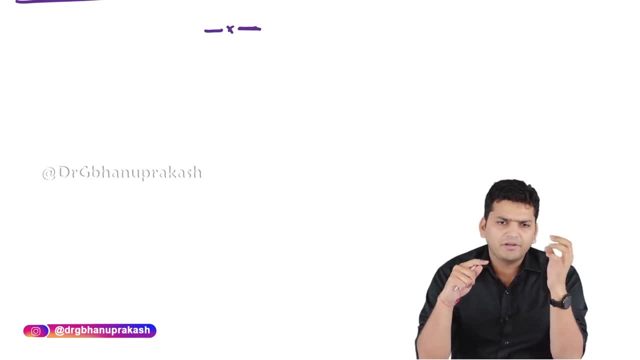 glucose. then we have discussed about the nutritional requirement: essential, semi essential, non-essential. then there are two special properties: one is the derived amino acid and the the aromatic amino acid. one for one point: I forgot to mention about the aromatic amino acid that you can write in the aromatic amino 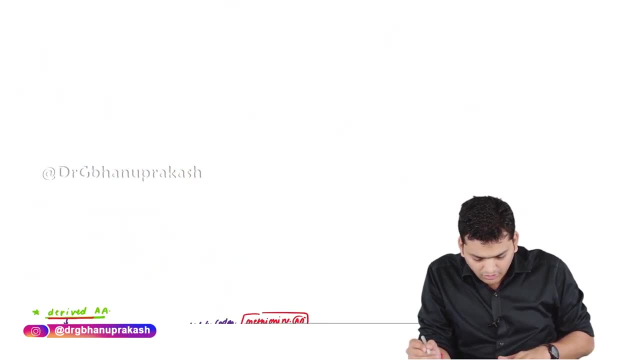 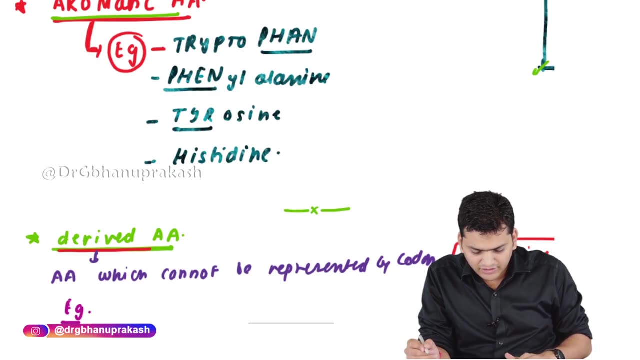 acid. if I just scroll up the thing, the nodes, we have written that in the aromatic amino acid. there are four examples: tryptophan, phenylalanine, tyrosine and histidine. you can write. there is one more point that you can write is: aromatic amino acid has a tendency to. 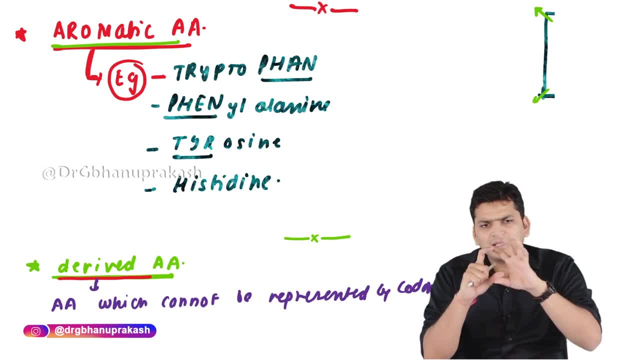 absorb the UV rays. they have a tendency to absorb the UV rays when you place these amino acid in the sunlight. sunlight can change UV rays, so these amino acid will absorb the UV rays. among these for this, among these, for the tryptophan is having the maximum absorption of the UV rays. so you can. 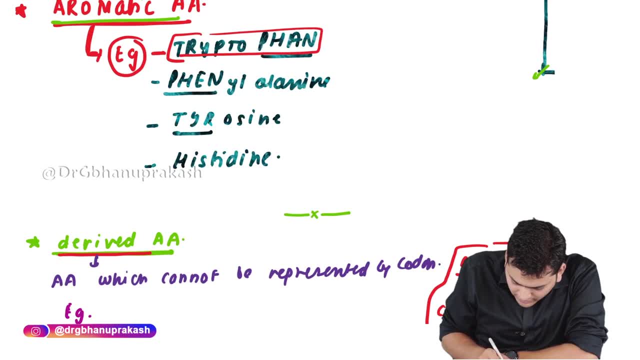 write this point here- that all the aromatic amino acid have a tendency to absorb UV rays, maximum UV absorption. maximum UV absorption is seen with tryptophan. this was asked in the exam earlier, that which amino acid has the maximum tendency to absorb the UV rays? the answer is going to be tryptophan, right. so all the aromatic 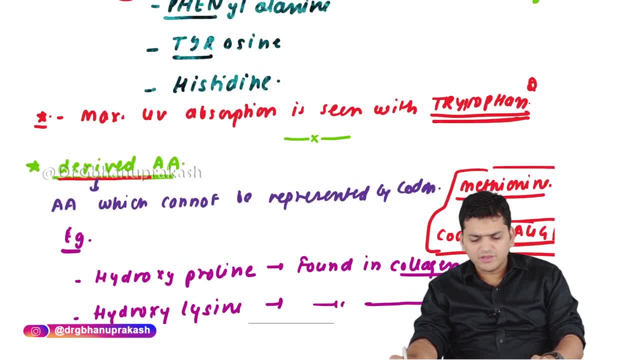 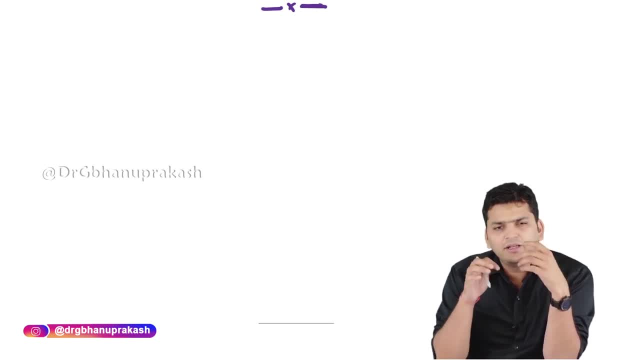 have a tendency to absorb the UV rays. the maximum is with the, the maximum is with the tryptophan, maximum is with the tryptophan. so this is the complete classification of the amino acid because, as I saying that earlier, we have only 20 types of amino acid. now we have added the 21st and the 22nd amino acid, so we 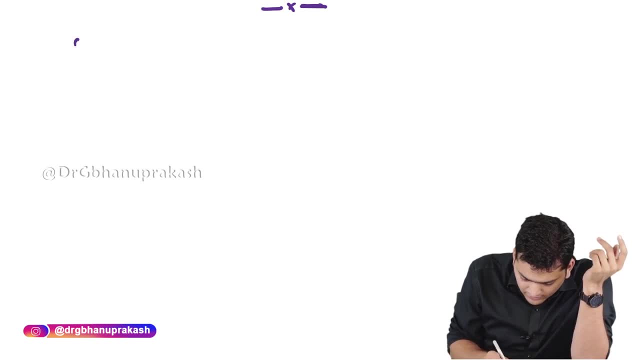 should know few details regarding them. one is the 21st amino acid. the 21st amino acid, the name of the 21st amino acid is selenocysteine- selenocysteine. if they ask that, what is the codon? 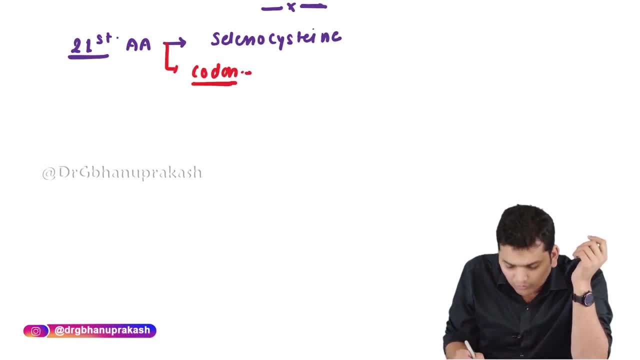 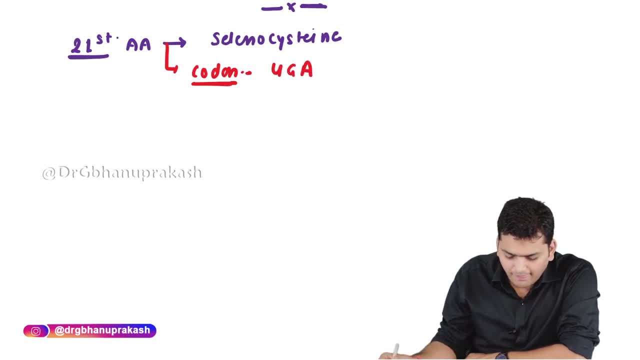 selenocysteine is UGA. if they ask that, what is the? the precursor? precursor amino acid means selenocysteine is synthesized from which amino acid? what is the precursor? the precursor is serine. serine will convert ultimately into selenocysteine. so the precursor amino. 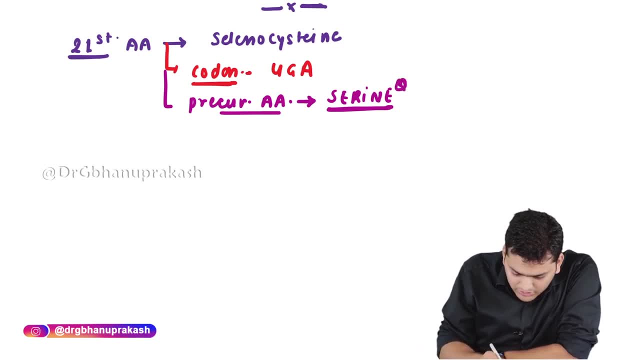 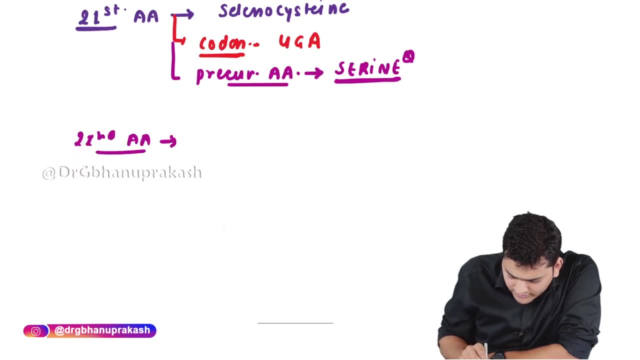 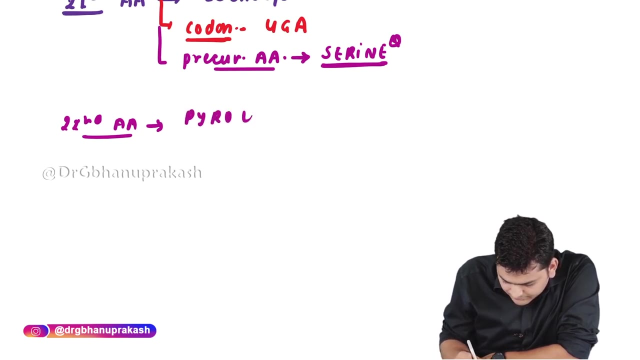 acid is serine is serine. when it comes to the 22nd amino acid, the example of 22nd amino acid is: the name of the 22nd amino acid is pyrolysin. the codon for pyrolysin is UAG. 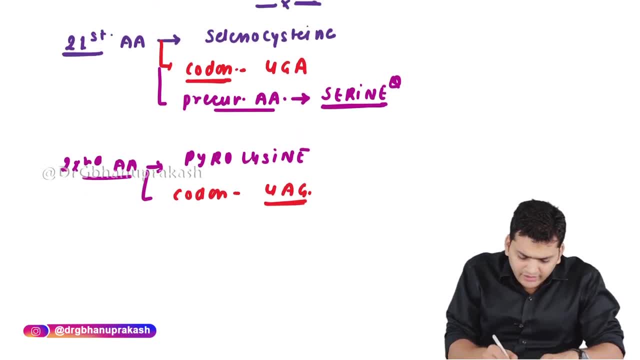 there is no as such precursor for pyrolysin, so the codon for pyrolysin is UAG. there is- These are the details to be remembered- for 21st and 22nd amino acid. 21st is selenocysteine and 22nd is pyrolysin. 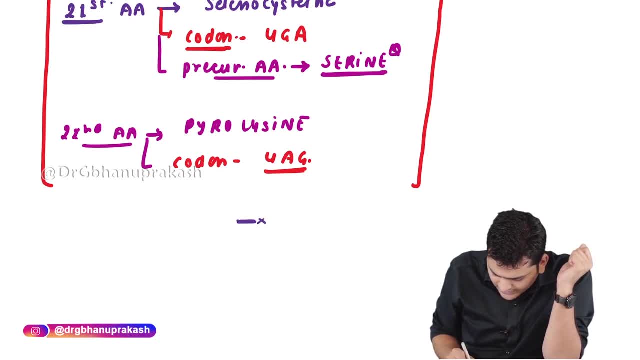 So, once we have completed this entire classification- this entire classification is a very important topic- There is going to be one question, 100% one question, from this discussion of the classification of amino acid.